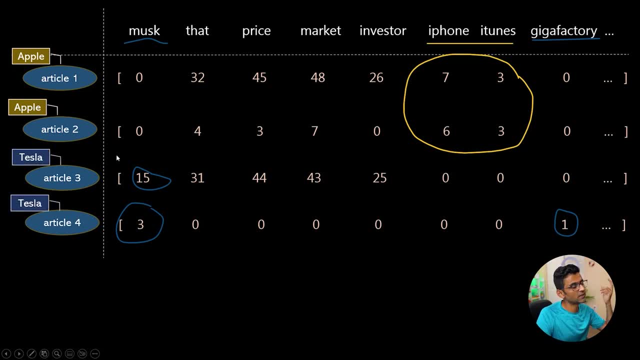 you can say, yes, this one is for Tesla and this other articles are for Apple. But look at these other terms that price market investor. Now these are very generic terms that can appear in any article. I used to work for Bloomberg and we actually were working on. 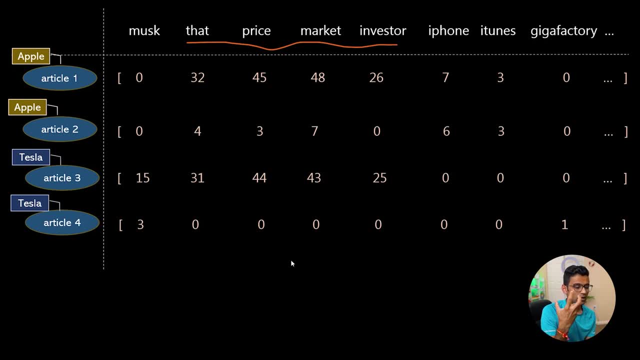 extracting company from earning estimate document And you will find this kind of generic terms too often in all the companies you know, like stock market, company profit loss. This and the presence of these terms in your bag of words model can suppress the meaningful words. 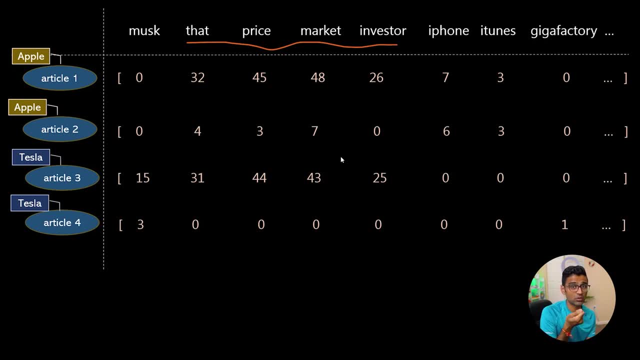 so here for i, apple, iphone, itunes is the relevant term and for tesla, musk and gigafactory are relevant terms. but these other generic terms are suppressing the influence of these relevant terms and in this example i'm just showing you four: that price market, investor, four terms. 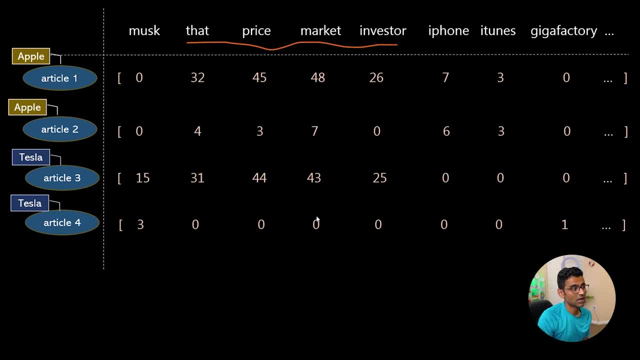 but actually there could be 100 such terms and look at what happens to the vector. in the first and third vector these terms are present with a equal amount, see 32, 31, 45, 44, so ignoring all the terms, if you just look at the vectors and you give this vectors to a computer, 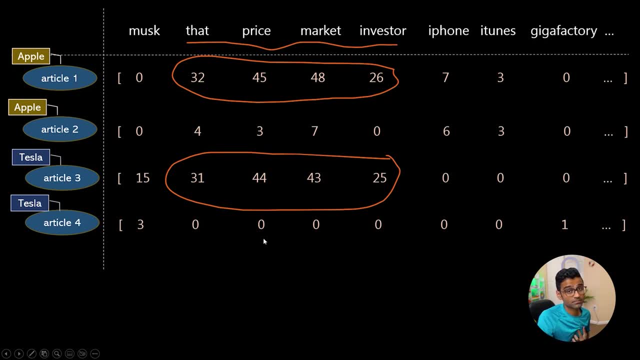 computer will think article one and three are similar. actually they are different. right, one is from apple, the third one is from tesla. but if you look at just the vectors, see this seven, three is not matching here, it's zero, zero. but see, other terms are kind of equal and there are four of them in reality. 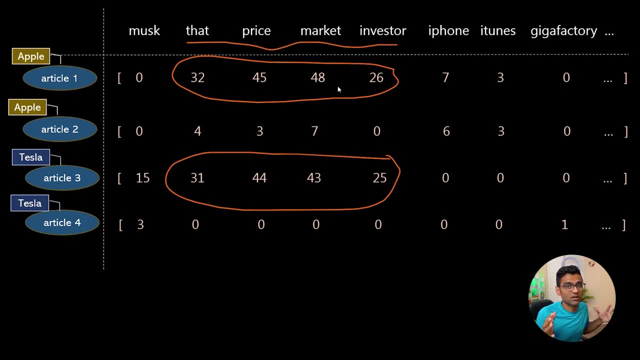 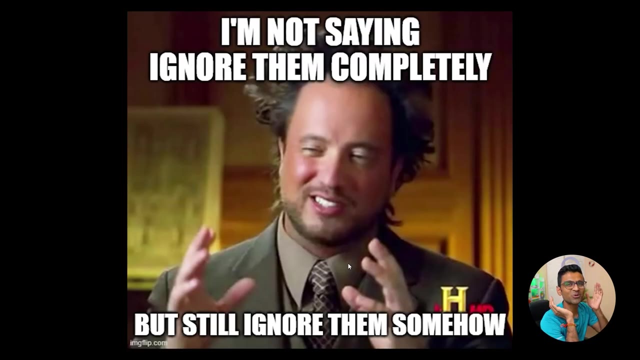 there could be hundred such terms in your vector and your computer will think: okay, these two are actually related articles, you know, but that is not the case. so how do you ignore these terms? that's the question. see, you don't want to ignore them completely, but still you somehow want to. 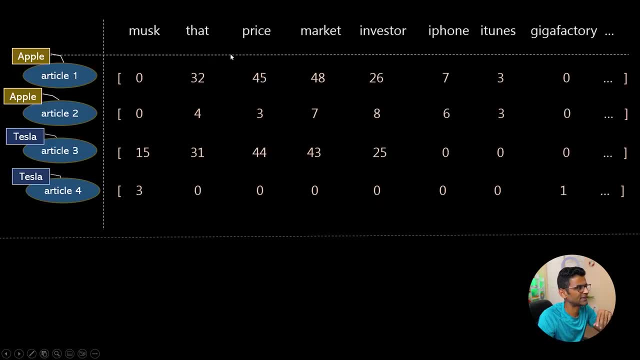 ignore it. someone will come and argue that, okay, that is a stop word. why don't we just remove all the stop words? fine, we remove that, but then how about all these terms? price market, investor? so stop words can help, but to a certain extent, we need to do some additional thing. so let's think about this together. let's pause this video. 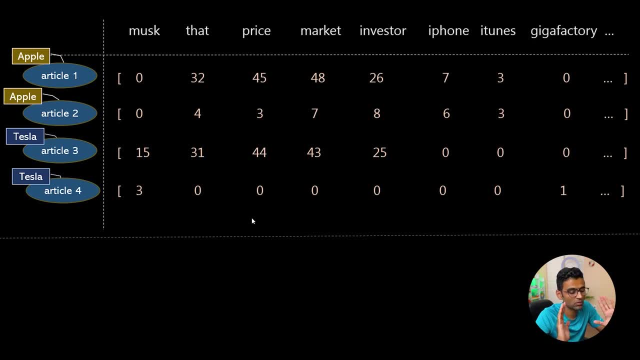 and think what can we do or what should be our approach. okay, you just pause the video and you will be able to come up with that idea. so one idea is we figure out in how many documents the term that appeared. so that appeared in three documents out of four, and i'm not talking about 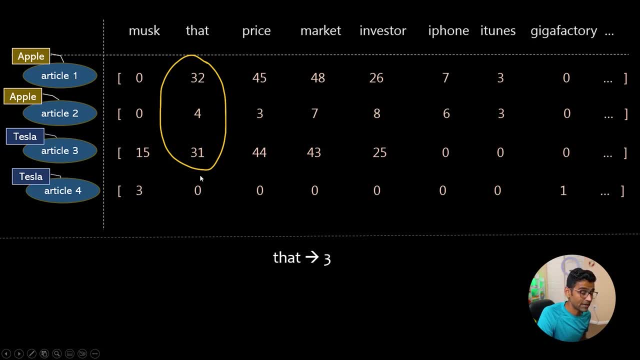 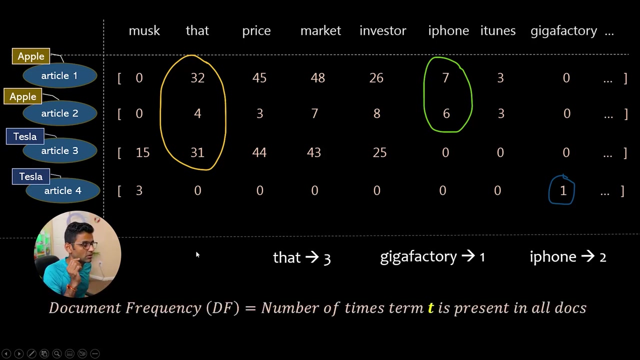 the individual word count in a given document. i am saying in how many documents this term that appeared. it appeared in three documents: article one, two, three out of total four documents. similarly, gigafactory appeared in only one document and iphone appeared in two documents. this is something called document frequency, number of times, term t. so t here is that gigafactory, etc. 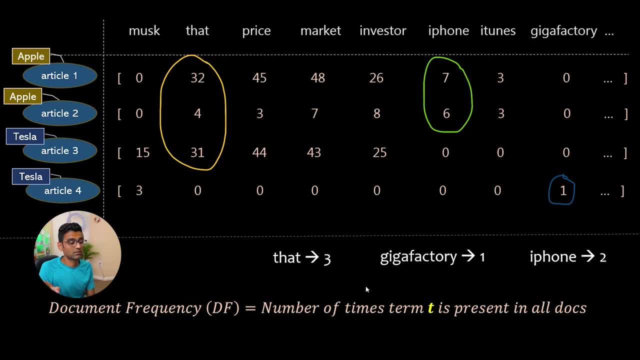 number of times term t appeared in all the documents, and if this number is higher, if some term is appearing in majority of documents, we should lower its influence because it's like a generic term, but if some word is appearing in only few documents, such as gigafactory, see only one. 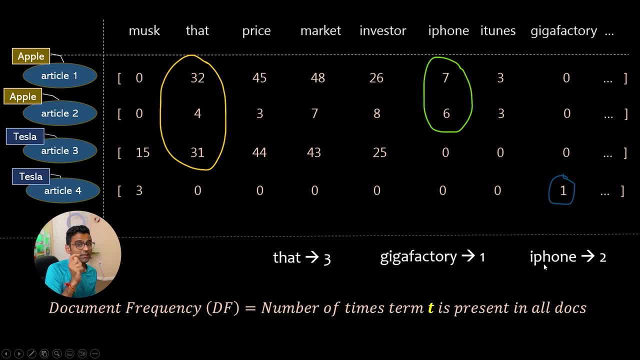 document: iphone- only two documents- then that term is important and we need to give it a higher number of times. term t appeared in all the documents, and if this number is higher, if some word is appearing in all the documents and if this number is higher, if some word is appearing in all the 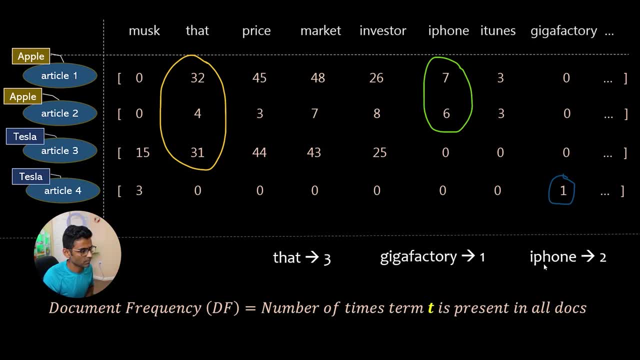 so we need to come up with some scoring mechanism here. and obviously the scoring mechanism should be such that you know, higher the term appears in all the documents, the influence would be lower. and you can do that by doing inverse document frequency. so if that term is three, so you invert it. 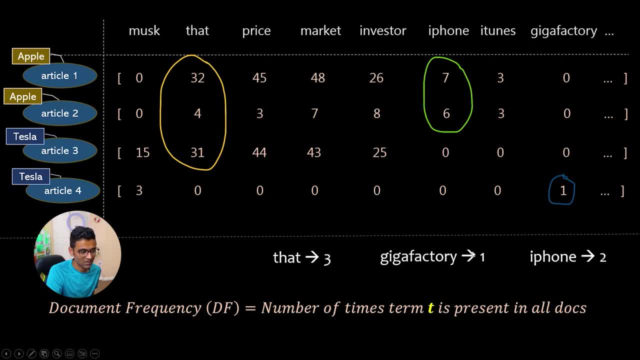 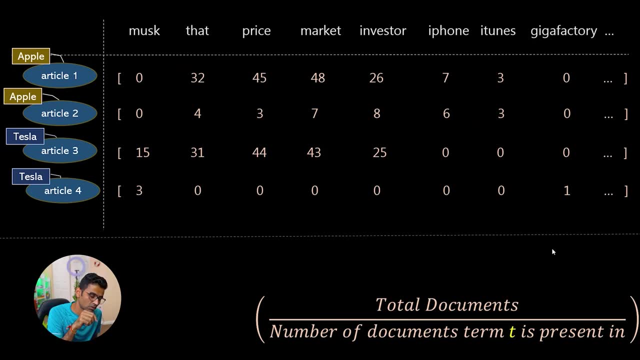 okay, then the number goes down and you don't do simple inversion but you do this formula: total number of documents divided by number of documents. term t is present in. for example, total documents are four, so numerator in our ratio is, is fixed four, but denominator is how many times that appeared in all the documents. well, three. 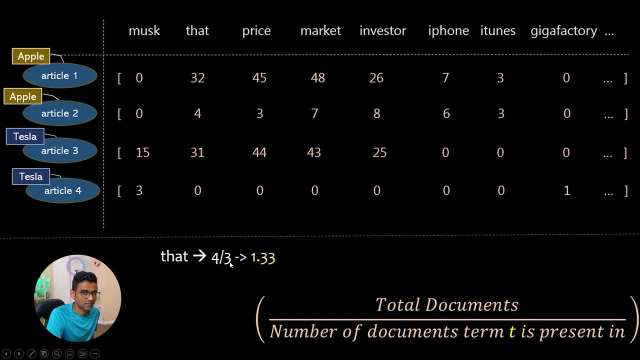 times. total number of documents is four. so if that's the case, then the number of documents are four. that appeared in in three documents, so 1.33. total number of documents are four. gigafactory appeared in only one document, so this number is four. so now see when the term appears in less. 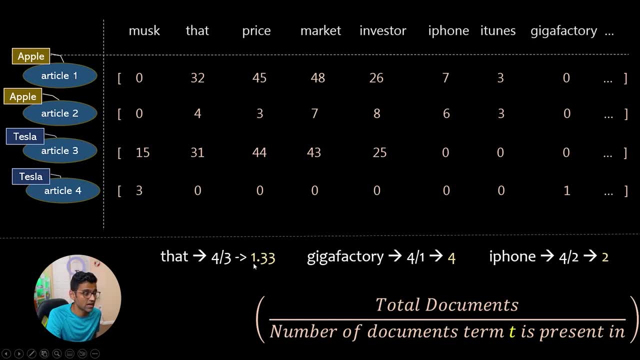 number of documents. the score you are getting is higher. see this, four is higher than 1.33, and this is called idf- inverse document frequency. there is something additional to this formula, which is called: you take a log of this. why do we take log? i will explain in a minute or so, but hold your thought. 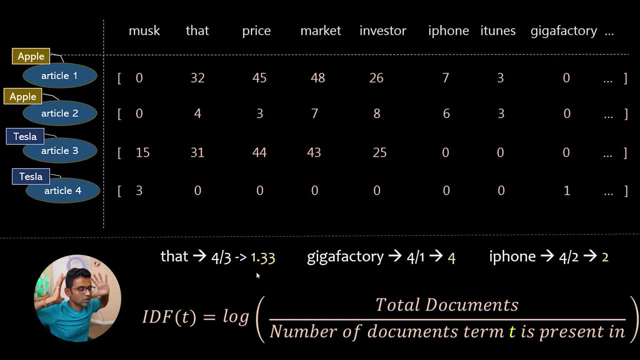 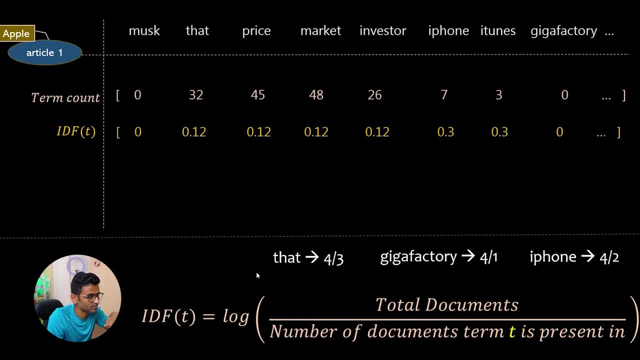 for now, and in your brain you should be thinking: if the term appears in more documents, the final score for that will be lower because you want to reduce the influence and you will come up with this kind of vector, which will be called ibf, vector 0.1 to 0.12 and so on. i mean, i, i'm just 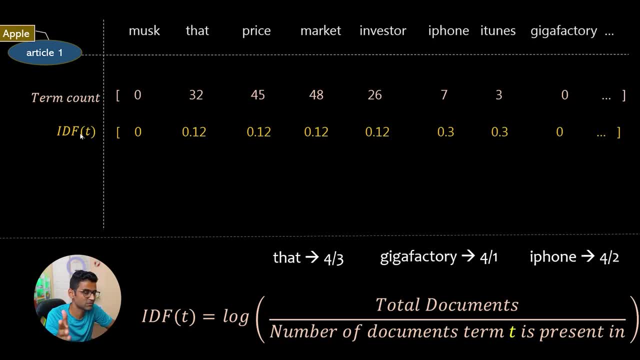 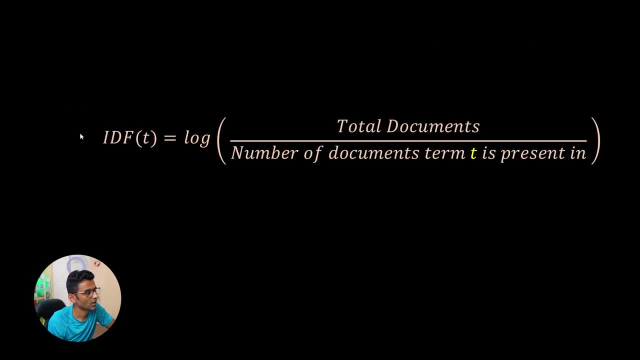 just showing this. we don't use idf, we use tf, idf, which i have to still explain, but for now, i hope the concept of idf is clear in your head. we also need to take into account the word frequency, because that is also important, correct? but we don't want to just take a word, frequency, like. 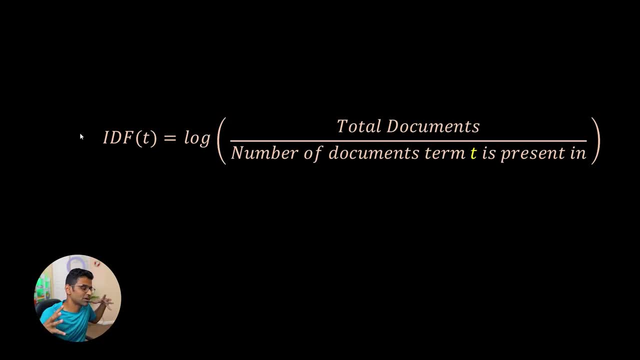 bag of words because see, some articles could be bigger. let's say there is a 5000 word article and there is only 10 word article, small article. you want to be fair and kind of normalized thing. so what you should do is total number of time. term. t is present in document, which is just a. 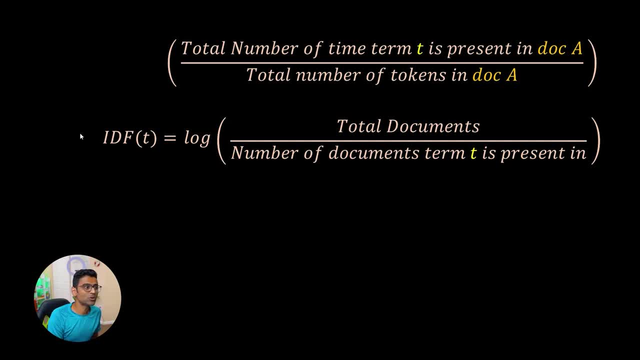 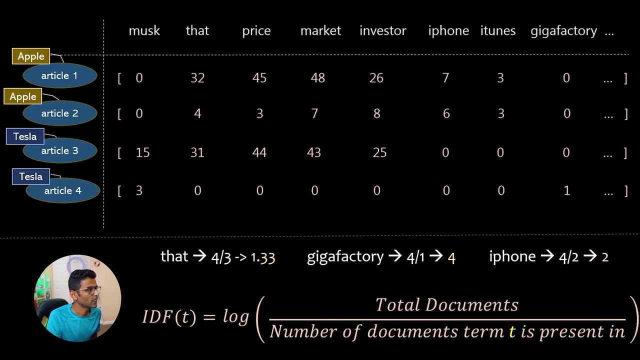 simple word count that we took in bag of words, model divide by total number of tokens in that document and that we will call term frequency. so here t is the term and d is that document in which you are counting that term frequency. so here, for example, the term frequency in article 1 for the term market will be 48. 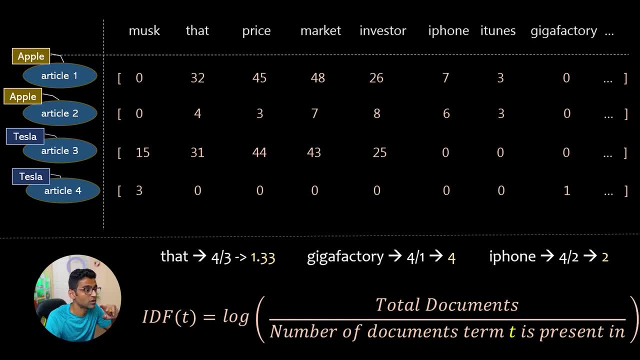 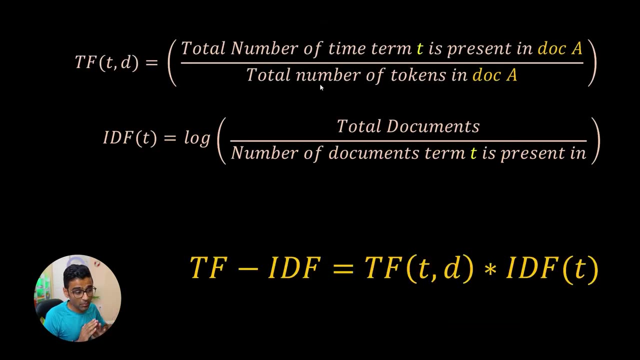 divided by total number of words in that article. let's say in that article total number of words are 1000, so the term frequency for market in article 1 will be 48 divided by 1000. and tf idf is just a multiplication of these two terms. 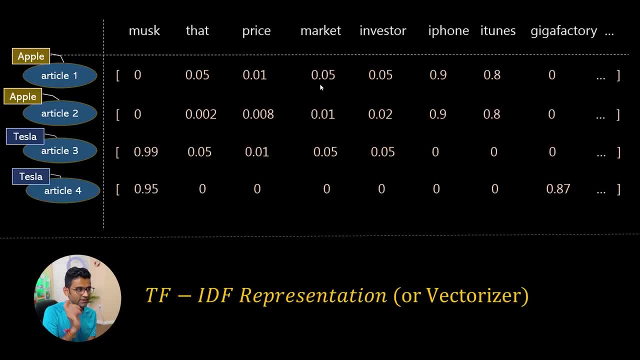 and we will use that in today's tutorial to do our coding. so we'll do again a text classification for e-commerce goods and we'll be using tf idf representation here. i'm just showing some sample numbers. i did not actually compute it, but what i want to show you here is terms like iphone. 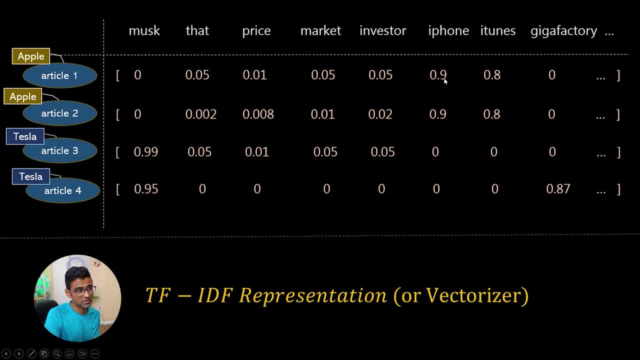 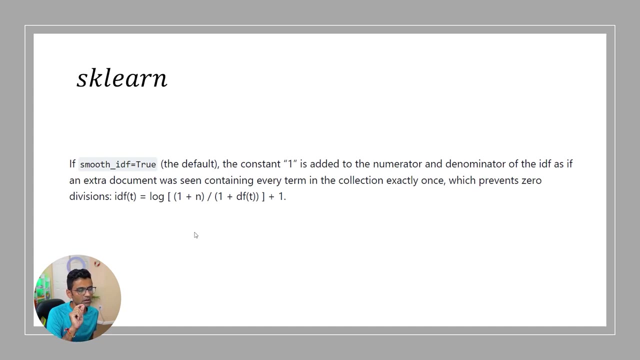 itunes gigafactory will have higher numbers- 0.9.8- whereas if you are using tf, idf representation terms like that price will have lower number. okay, one more thing i want to clarify is sk learn uses slightly different formula for idf to take into account the zero division possibility. so what they? 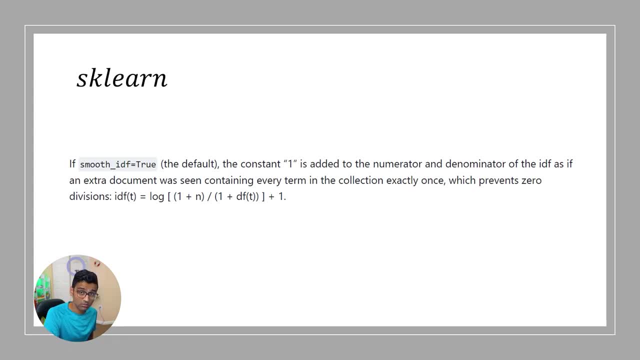 do is they add constant one in numerator and denominator both, and then the result they add one more time. so it's just a little customization on your idf formula. and then you can add more and then the result they add one more time. so it's just a little customization on your idf formula. 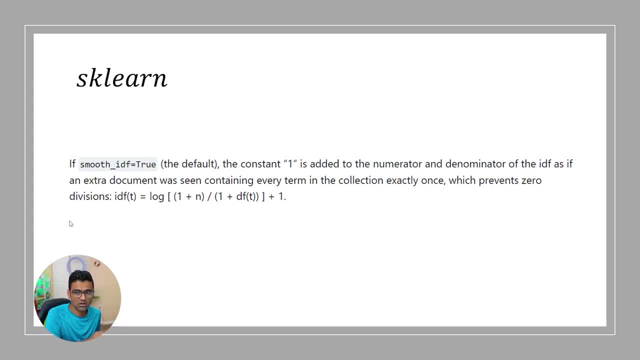 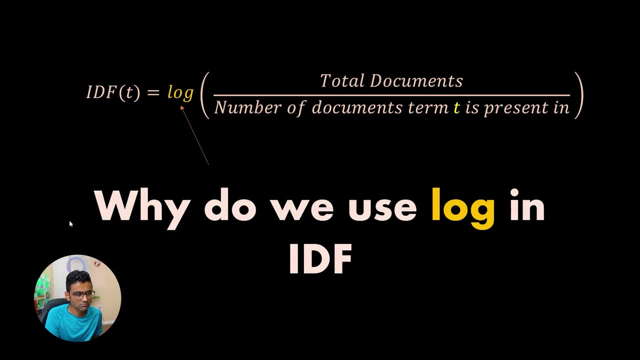 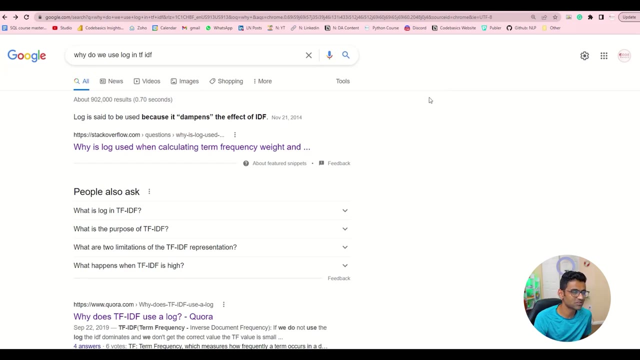 sk learn uses that. this screenshot is from the sk learn documentation. now let's talk about why we used log. you can ask this question to your dear friend who is sitting next to you, and that dear friend is actually google. so if you just google this question, you'll find the 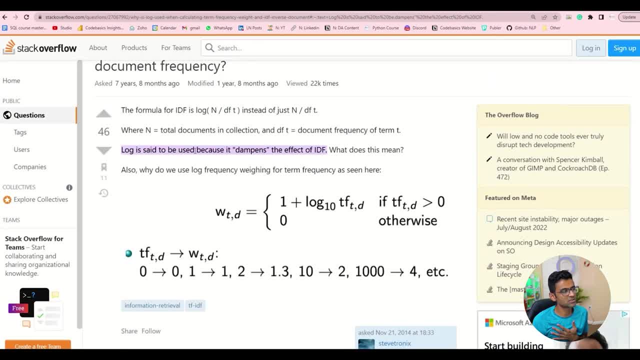 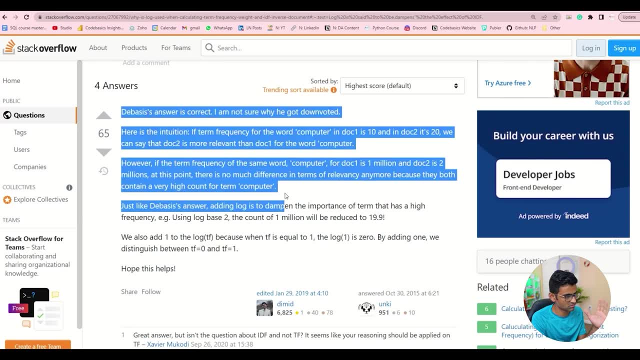 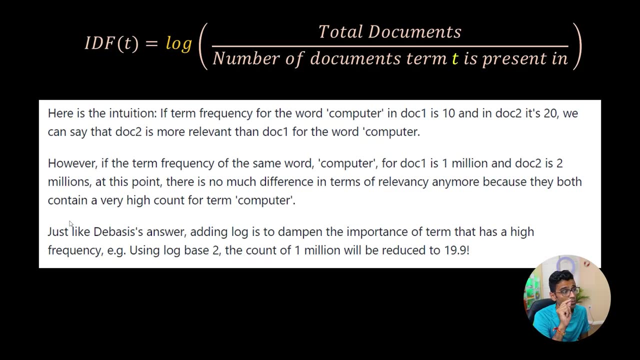 stack overflow answer where they say that log is used to dampen the effect of idf, and unki has given a very nice answer here, so i'm just going to take a screenshot of that answer and show it here. credit goes to unki and stack overflow, which is, let's say, in a in a document you have a term called 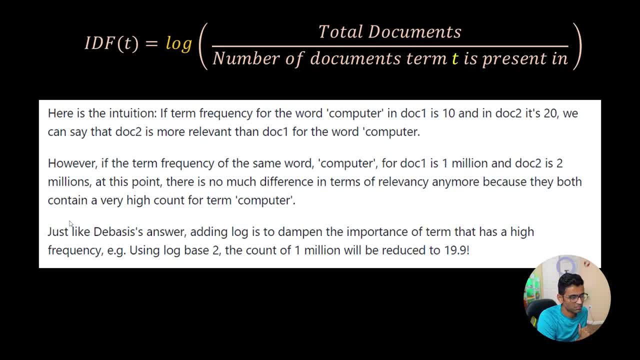 computer which is relevant for your given mlb problem, and if the term appears one million times, you know that that term is important and and i'm talking about that one term appearing in your document, right in your specific document. so now, if it is 1 million or 2 million, it is all same, correct, doesn't matter. so that's why we kind of 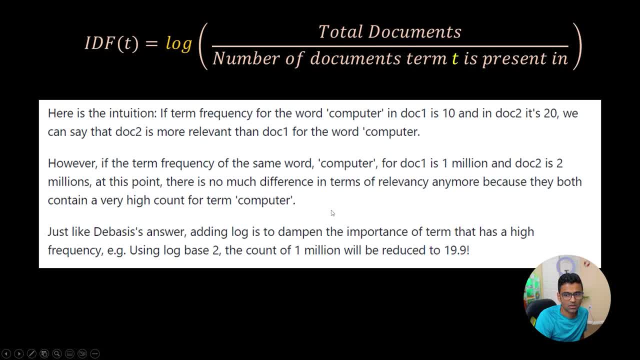 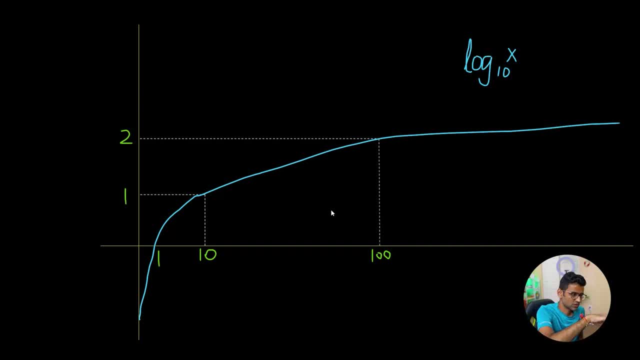 take a log of that just to kind of reduce the effect of it. if you know from your log function. your log function goes something like this: you know, log of 1 is 0, log of 10 is 1, log of 100 is 2. 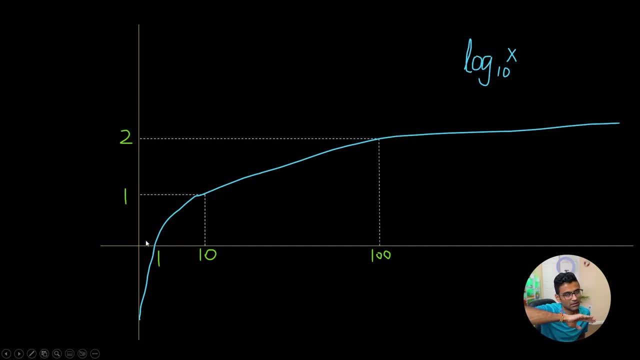 i'm talking about log to the base 10 and the call kind of flattens out as you go further in your x-axis and the influence that you want to have in in terms of your idf. you want to reduce it because as you have more terms the effect is same, so you can just reduce the influence. now 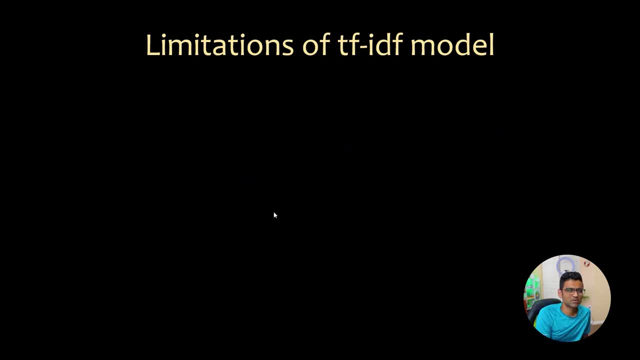 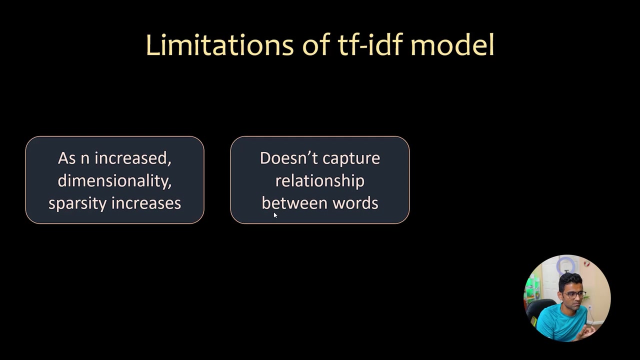 the limitation of tf. idf model is similar to the previous model that we saw before, which is: as you increase dimensionality, the sparsity increases. as your vocabulary increases, obviously the sparsity increases. it's a discrete representation of your text. it doesn't capture the relationship between the words. the relationship between the word is captured by: 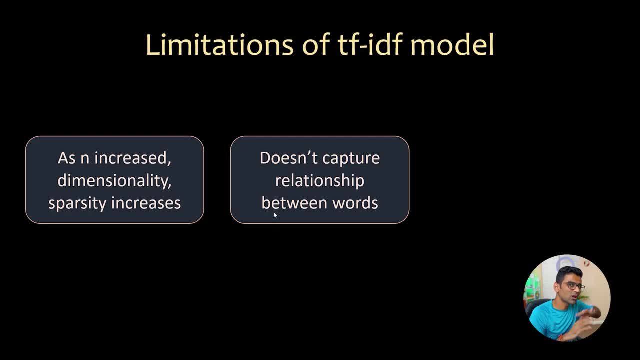 word embeddings and sentence embeddings, but all other models. they suffer from this problem. where you have relationship between the words, it's not captured because here you're taking a term and you're just taking a count out of it, and it suffers from out of vocabulary problem as well. 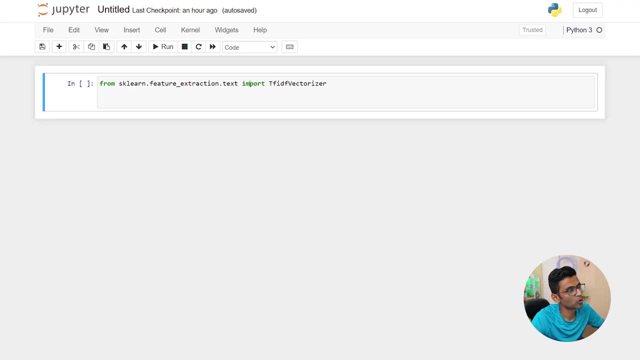 let's do some coding now. i opened jupyter notebook and imported tf idf vectorizer from sk learn and i'm going to take one sample. corpus, and the meaning of corpus is the collection of documents in your application. i'm just going to take some simple dummy sentences and will create tf idf vectorizer. 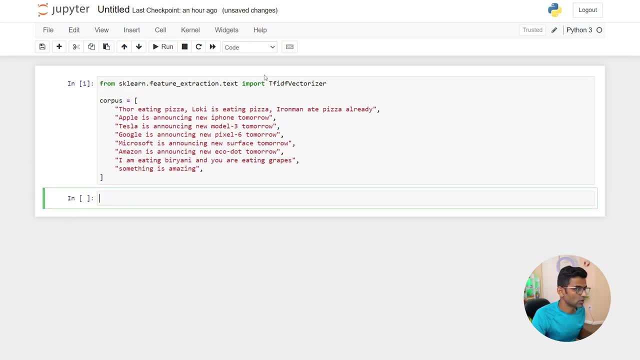 out of it. so the way you create the instance, this is tf. idf, vectorizer is a class and you just create an instance of it and you will just say fit. so when you do fit, you are creating that vector, basically right. and then you're kind of training basically, and then 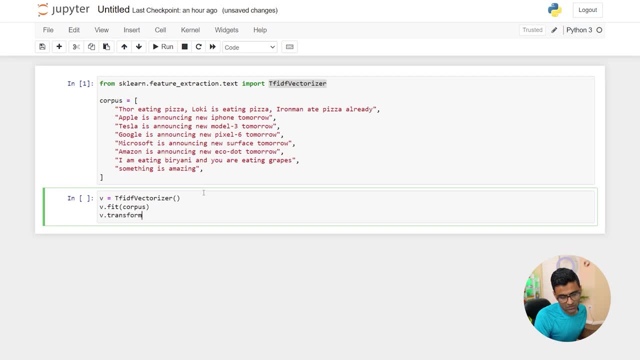 the creation happens. when you say transform, you can do fit, transform as well. just one call. i think let's do that fit and transform and we'll call it transformed output. is that okay? and once that is done, the v object will get its vocabulary. so i want to print. 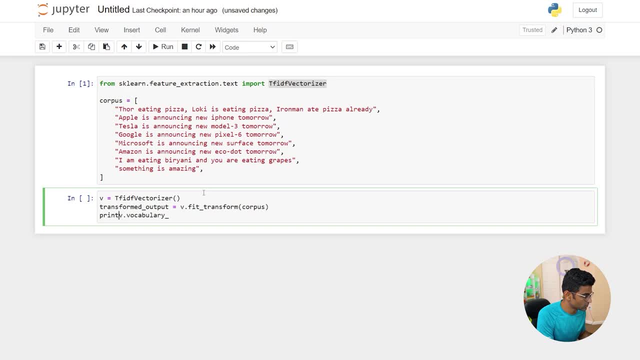 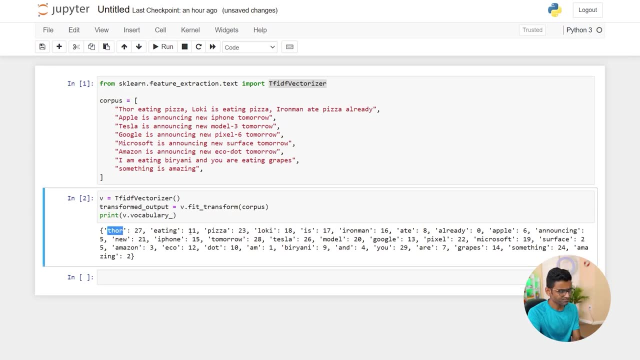 a vocabulary first and i'll just use print so that i can see everything in like two or three lines. see all this vocabulary. have these indexes for example, already, the term already is at zero, apple is at six, and so on. now i will print idf score. so v this parameter, v, if you do like dirv you. 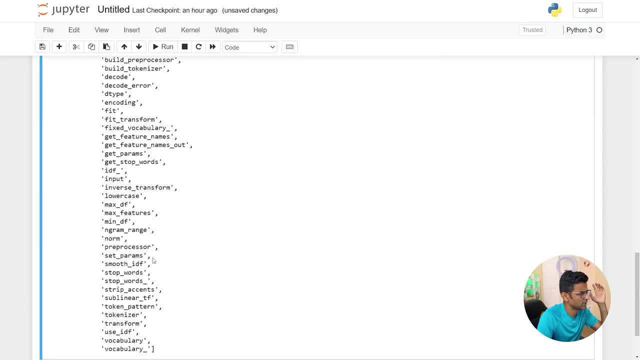 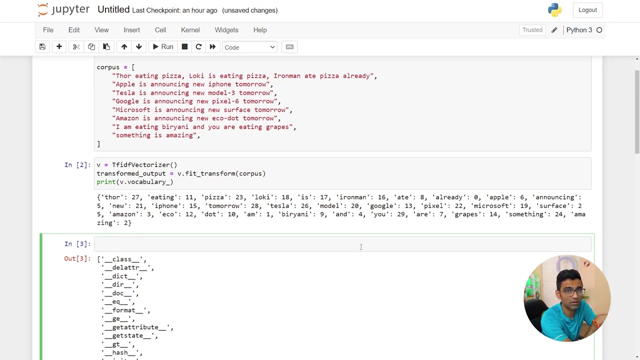 will see all the members and you will see idf, for example, as one of the members idf smooth idf. actually we are using smooth idf and so on. so let me first print just a simple idf score out of it and for that you can either iterate through this particular directory- uh v, dot, vocabulary- or, if you want to go, 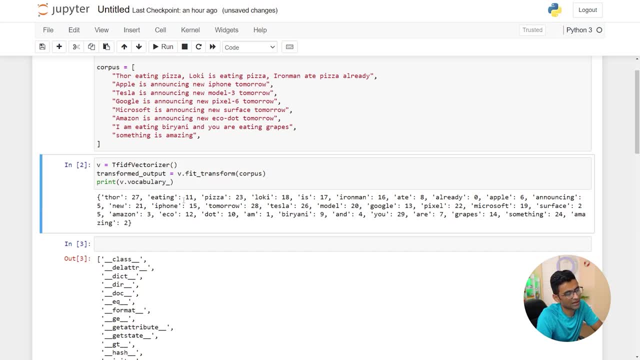 in sequence, see if i i i treat through it, this directory. i'm kind of going randomly over the places. but i want to go in sequence where i take the zeroth index element first and so on, and for that we can do v dot, get feature names out. 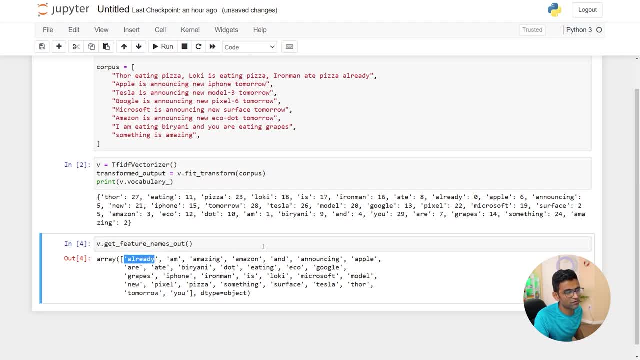 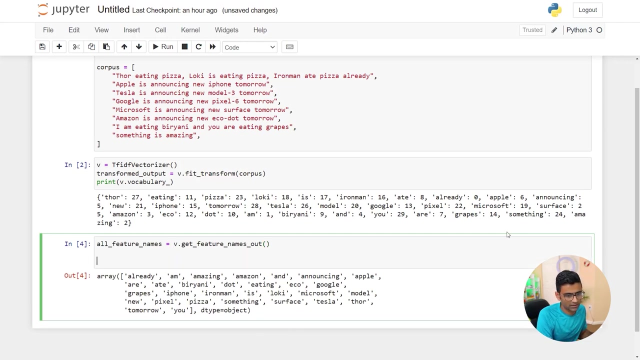 and that will print things in order. basically all your features, all your vocabulary, already zero, m is one. okay, when you do tf, idf, vectorization, these are actually your features and based on the features you will calculate your vector. so i will just call this all feature names and then i will iterate through it. so i will say for: 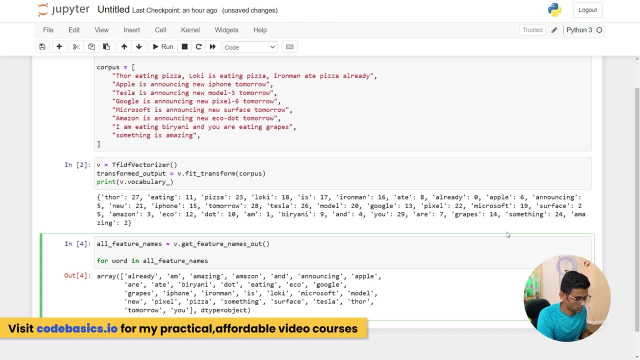 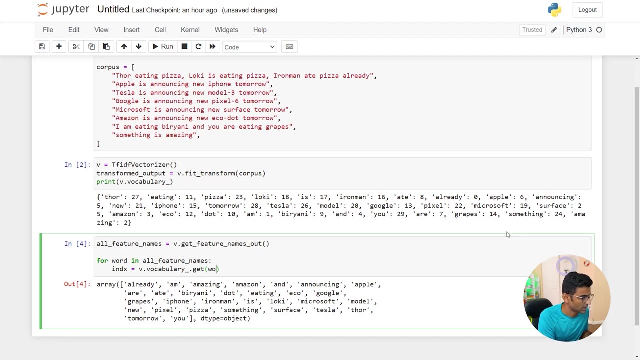 word in all feature names. i will first get the index, and index is v, dot, vocabulary, dot get. because it's a dictionary. you can call get method and you get this particular index right, like 27, 11, whatever, and when you get that index you can then say v, dot, idf, that will have your idf score and you can retrieve specific. 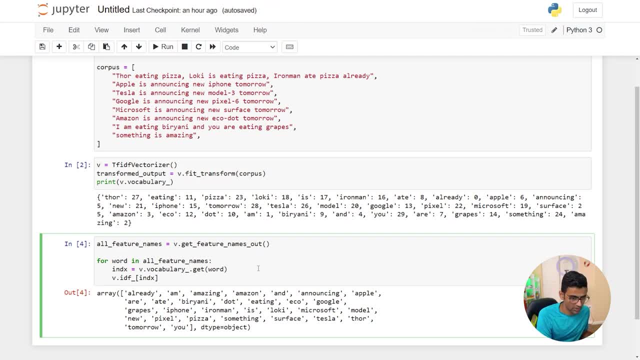 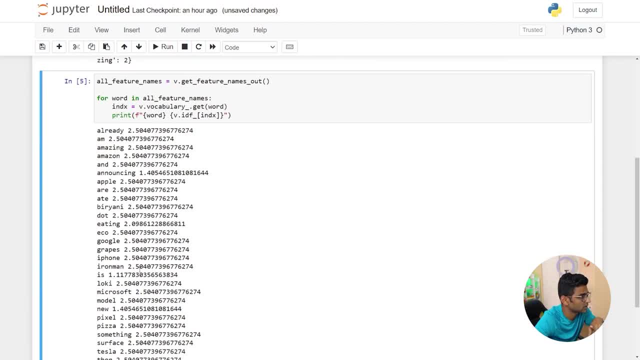 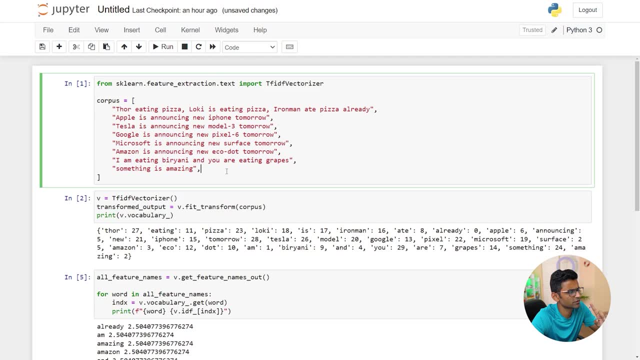 okay, so this is the score. now you will notice one thing, which is this term is is present everywhere, see, in most of the document it is present except this one. so you expect the tf, idf or let's say idf, score for is to be lower and the term like apple. 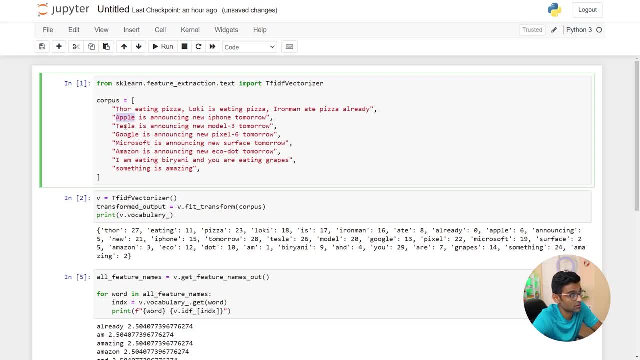 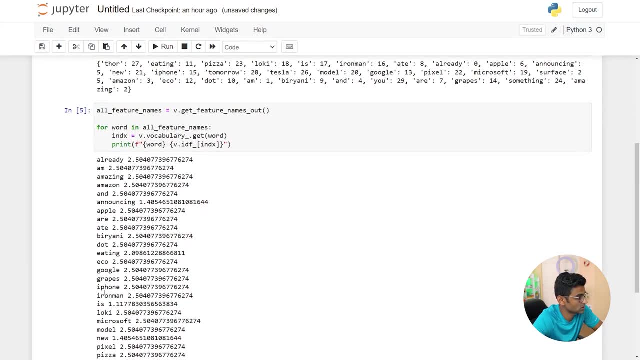 is appearing rarely. so the score of apple, tesla etc. should be. it should be higher. so check this: is is 1.1, whereas amazon or apple is 2.5. so it is working and we are more interested in the the whole tf idf score. so what i will do is now i will print that. 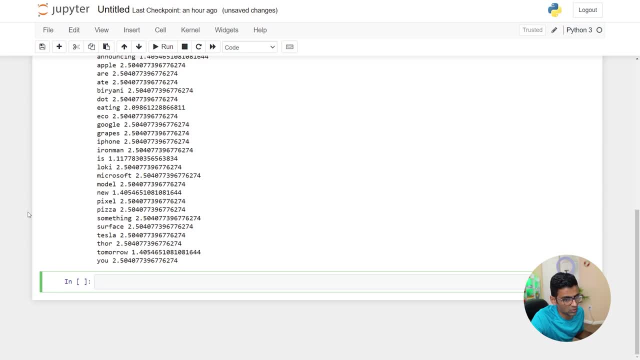 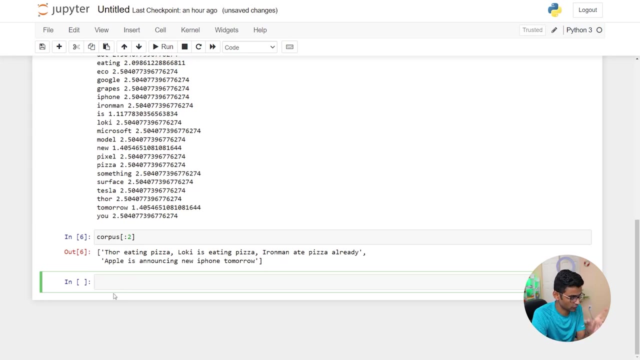 and that score is present in transform output. but before i do that, i will let me just print first two sentences from the corpus. okay, so these are the first two sentences from the corpus and i want to print the corresponding tf idf vector for these two sentences so that that is present in transform output, correct? 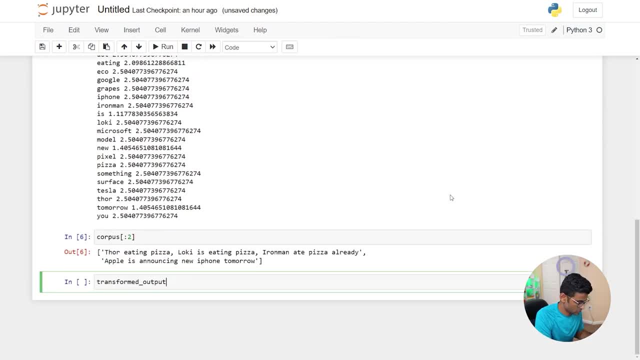 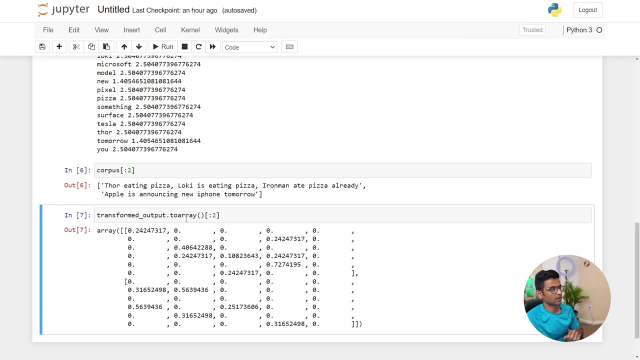 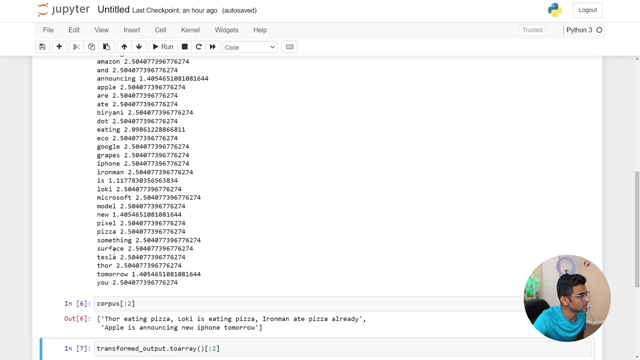 we got that in transform output. so transform output, dot to array. it's a sparse matrix so you have to convert it to an array and you just do two. so this is the first one and this is the second one. now watch this. uh, let's see we are looking at, is okay and is. 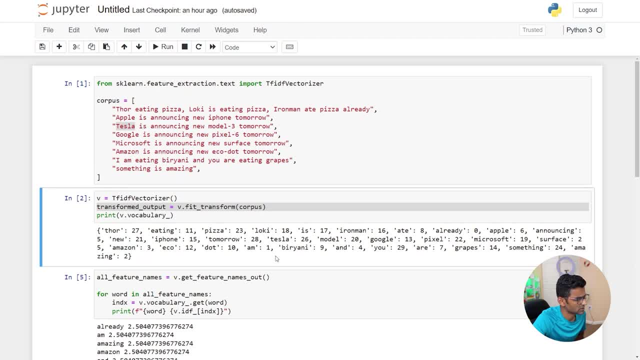 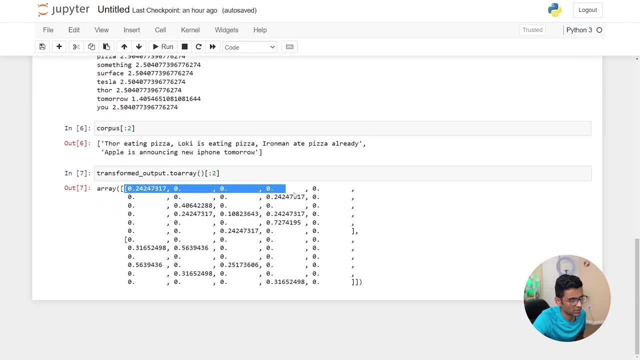 is at, i think, position 17. right, so is. if you look at it here, it is 17.. so is position is 17.. so there are total six here. so the position 17 will come. uh, let's see where. so six, six. so this will be zero, one, two, three. okay, zero one, two, three, four actually. 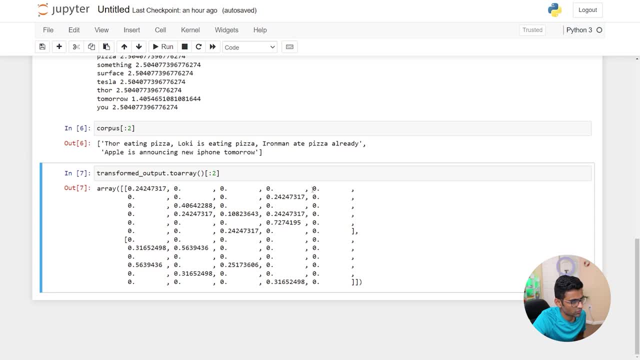 there are only five, i see, so this will be 15, 16, 17, it will be this one, i think this one actually, oh see, zero one, two, three, four, five, six, seven, eight, nine, ten, eleven, twelve, thirteen, fourteen, fifteen, sixteen, seventeen, so see the idf, tf, idf, score for. 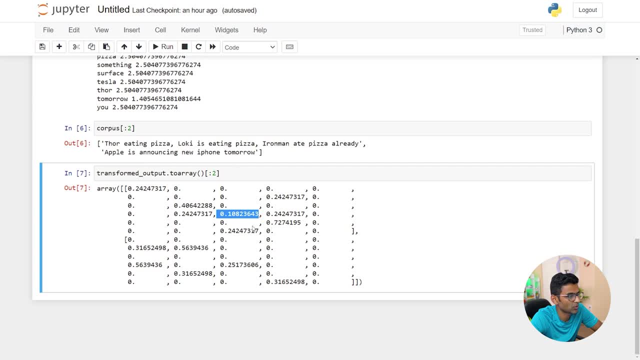 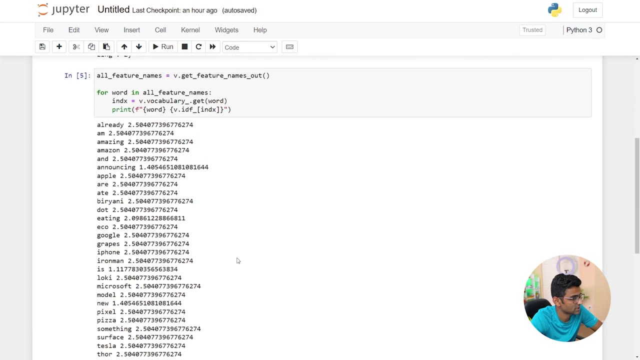 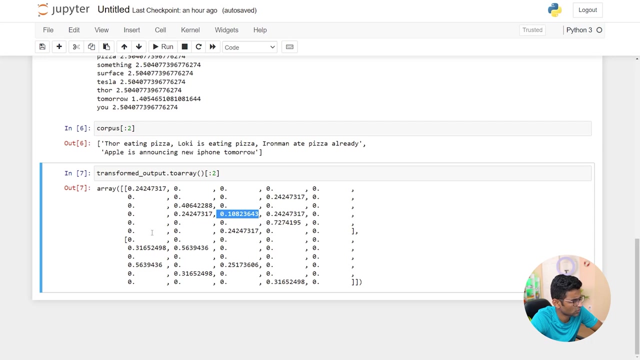 is in the first sentence, is 0.10, and the score for thor, for example, is: how much. so where is my thor? thor is 27, so this is 17, 18, 19, 20.. one, two, three, four, five, six, seven. see, thor's score is 0.24, so it is more than is so just. 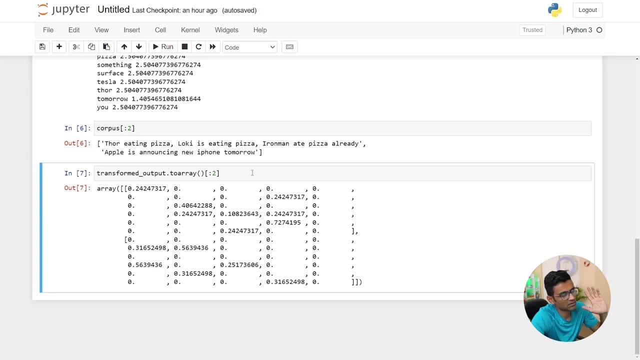 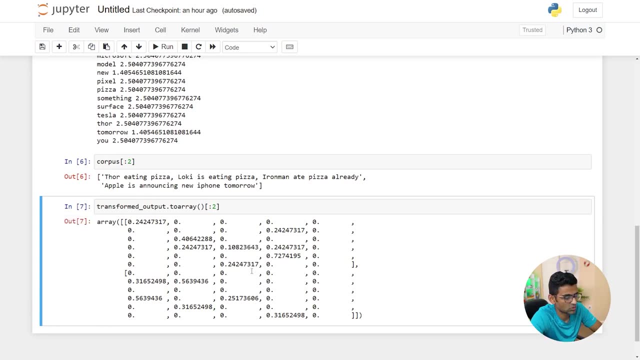 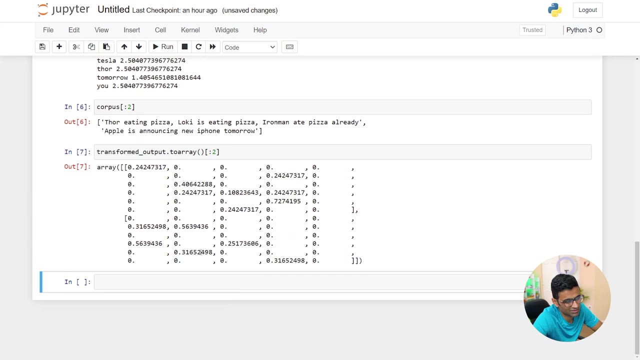 consume this, i mean you'll get an idea that the things are working as expected. the score for the term which is appearing in too many documents is lower and the score for the rare terms which appear in individual document is higher. i mean, that's. that's the whole point i wanted to make. 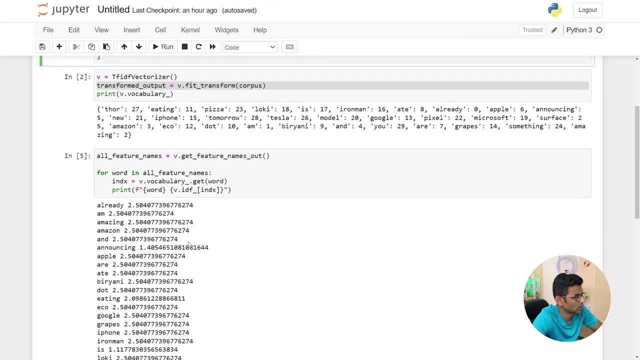 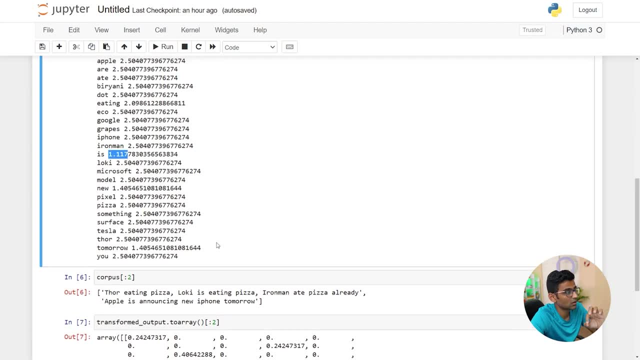 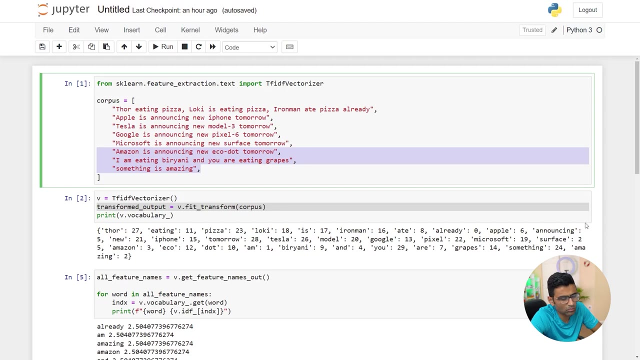 if you remove certain sentences, for example, right now, the score for is- idf score for is- is 1.11. if i remove certain sentences, you'll notice that the score will go up. you can experiment. we want to move to our actual problem. that will be solving in this coding tutorial, which is: 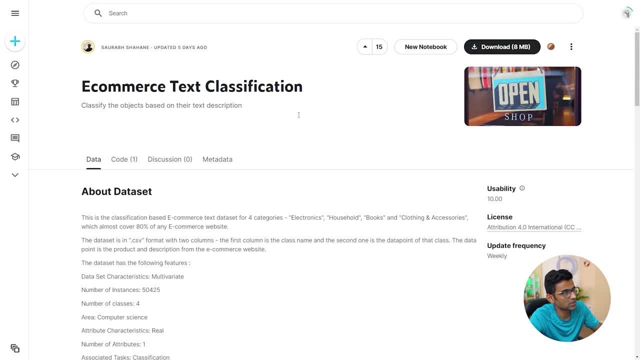 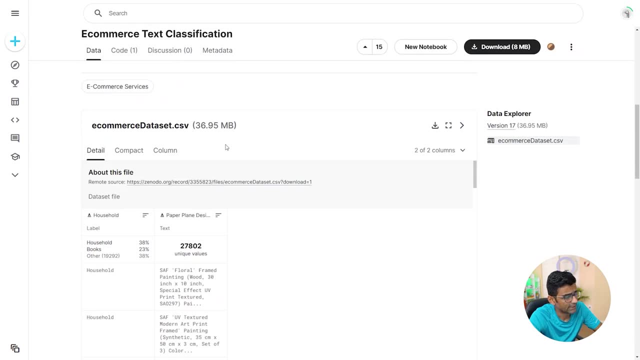 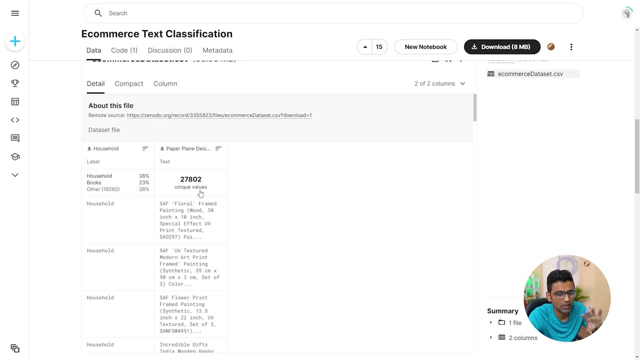 e-commerce text classification. okay, and i took the data set from kegel. the source credit is going to: source credit is given to this particular page. this data set has four classes. i mean, the actual classes might be more. i have trimmed it down and we have the description of an item that you sell. 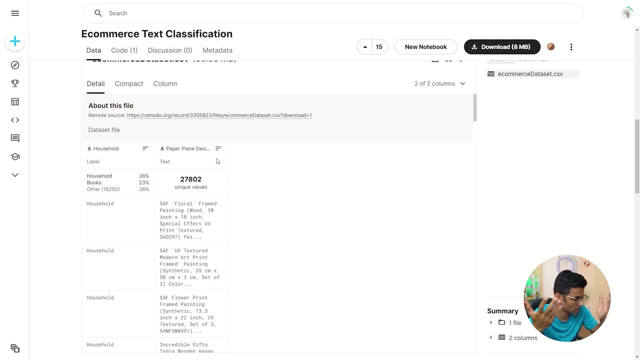 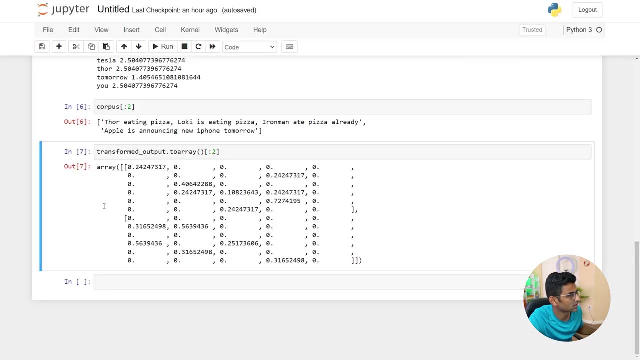 it on, let's say amazon. so amazon item description, amazon or any other e-commerce website- item description. and what category is it? electronic, household box, etc. okay, so it looks i have. i have this other notebook that i usually prepare before my coding video. so see, it looks something like. 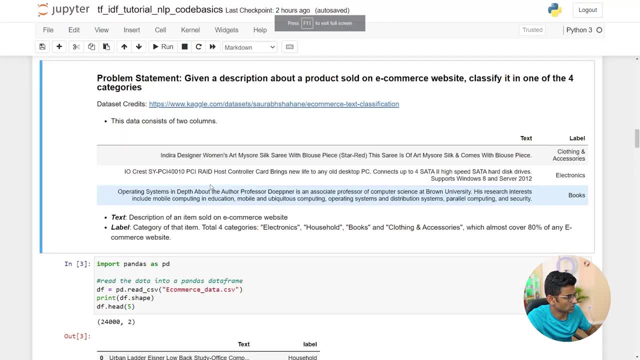 this you can see right. so let's say there is a text and there is a label. there is a text, this text, when you read it you realize it's electronic, right, sata, hard is drive. and when you read this one you realize it's a book. 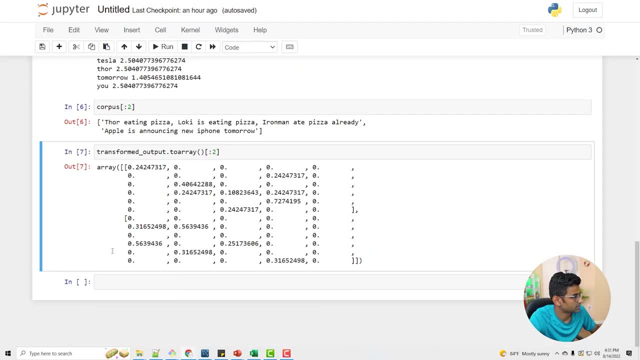 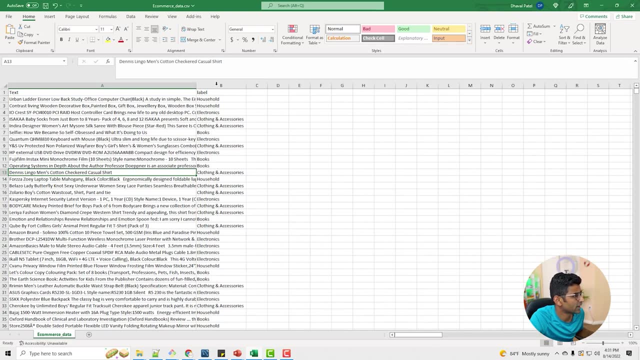 so we have this one and what we want to do now let me just show you the csv file. so i got the csv file. number of categories are total four. okay and see, these are the text description. so simple csv with two columns: the description of an item and what category that item belongs to. 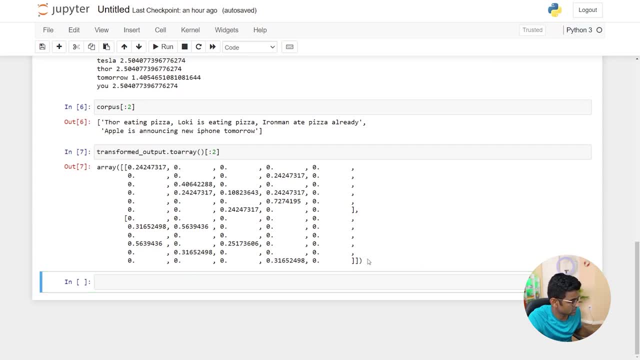 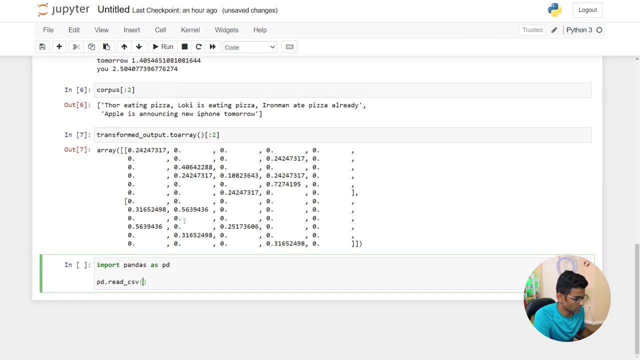 okay, so let's import pandas. so how do you import pandas? import pandas as pd. how do you read csv? we have done this like i don't know 10 000 times. so you read ecommerce cv, you store it in your data frame: df dot shape. you can print that and then do df dot head. 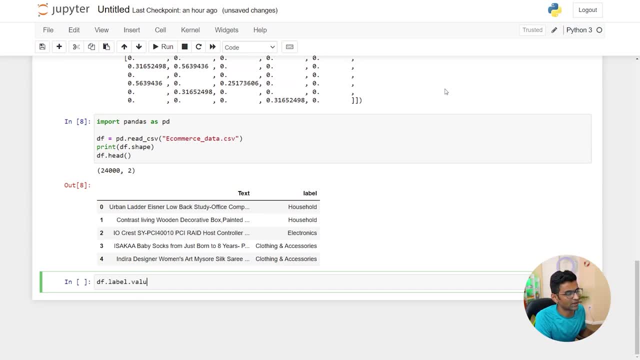 what i do is i usually do f dot label, dot value count just to check if it's correct. you can do flabelvaluecount just to check if it's correct or not. you can print that and then do df dot head. what i do is i usually do flabelvaluecount just to check if it's correct or not. 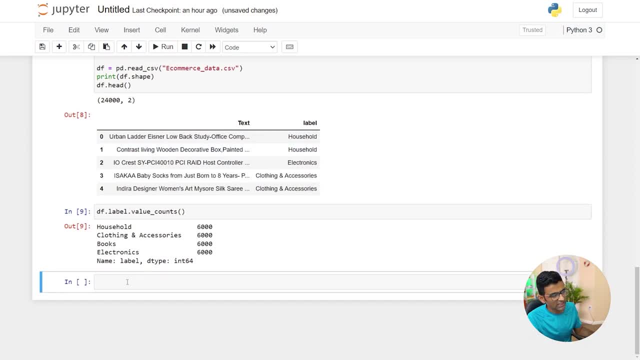 there is a class imbalance and no, there are six thousand items in each of the categories. as I said, like, I trimmed down the data set so that there is no imbalance, and now what we will do is map these label categories to numbers. machine learning models understand only numbers. so how do you do that? so df dot. 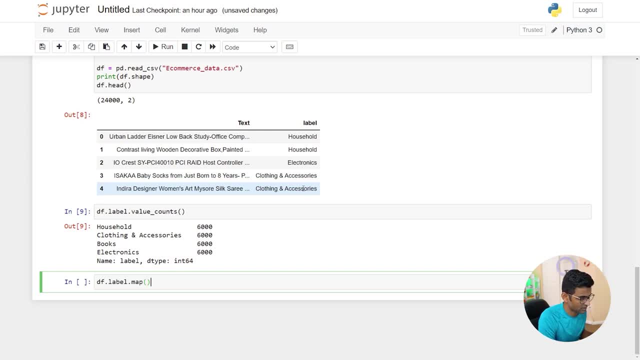 label dot map. you can use a map function and you can apply the dictionary mapping. so what you will say is: okay, if it is household item, map that to a number zero, just random number. you know, zero, one, two, three, four. if the category is books, the number is one and so on, and that will be my label number. 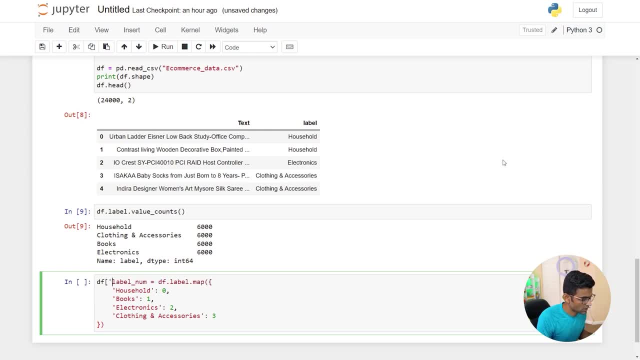 column and the way you do that is you'll have to specify the new column like this: this is a new column that you're creating in pandas. pandas is an awesome library. you can create new columns like this by applying transformation on existing column, and I will check my DF head and it works like. 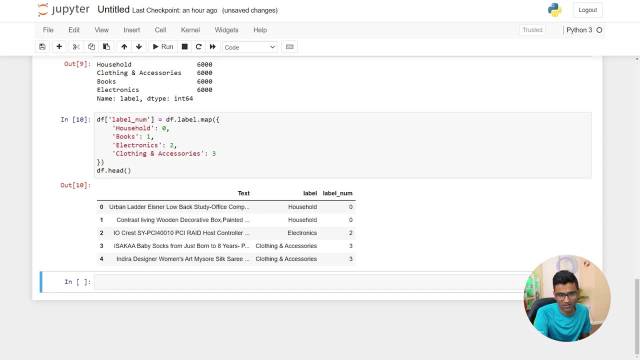 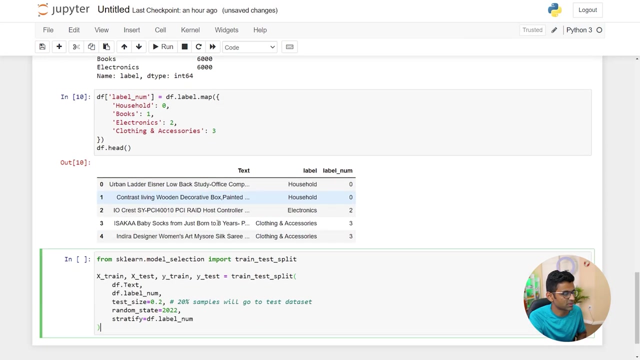 a charm. okay, we are ready for train to split as usual. this would be in your muscle memory. import it from sklearn. the train test split method and we have done this so many times that I don't feel like writing it, I'll just copy paste here you. 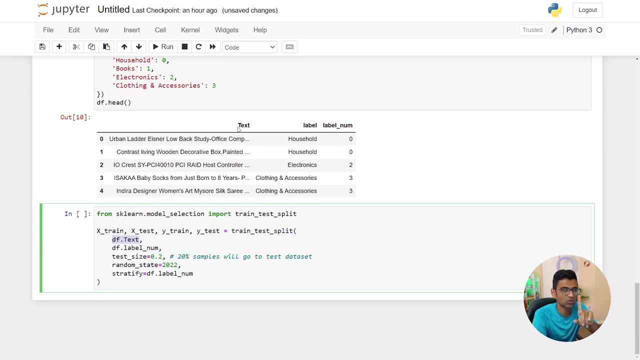 are doing train test. split off. df dot text is your main, actually it is your dependent variable. and df dot label number is your independent variable. it's like a target variable, correct? so this is x test, x train, this is y test, y train and this is the split train and test into 80 percent, 20 percent category, 20 percent. 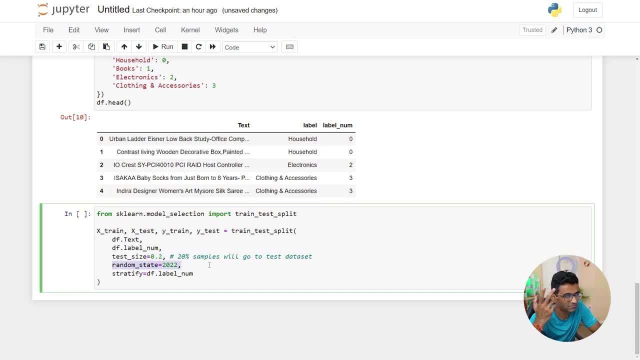 samples. go to test data set: random state parameter. I'm just randomly initializing it to num some number and then we are doing stratify. actually, if you don't do stratify, still okay, because no, actually we we have to do it. okay, otherwise you might get imbalance in your x train extra. so this is a good practice and when you do that, 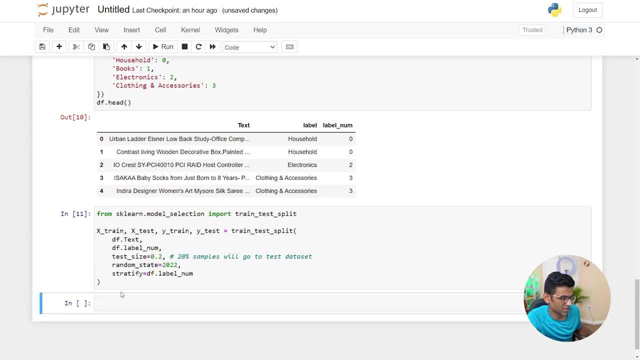 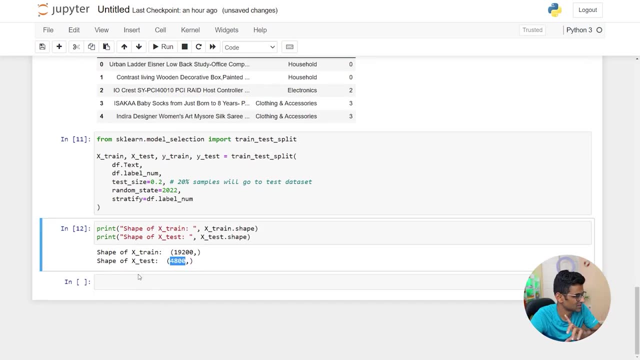 you can do train test split and I'm just going to just print the shape of x train. x test took something like this: 4800 samples in your test data set, okay, and then just some value checking in in your y train. I'm doing value counts and you can see that there is a balance. you 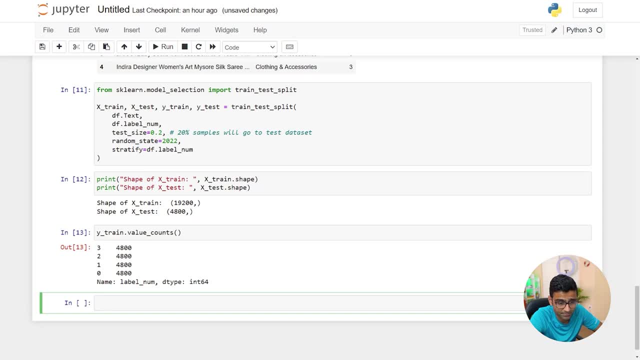 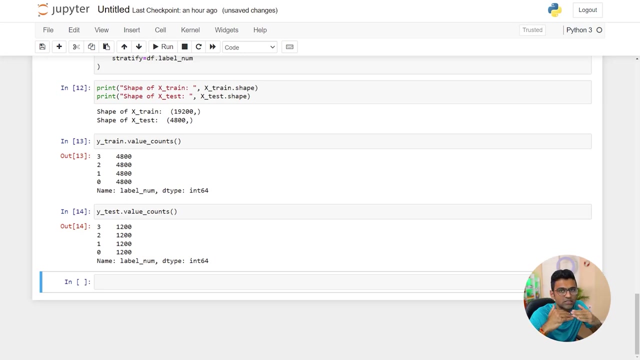 know every category has 4800 training samples and same thing you can do for y test, right? so y test value counts and y test also has equal number of samples from all the categories. now I will use few classifiers from sklan to train my model. I'll first use k and then random forest. then 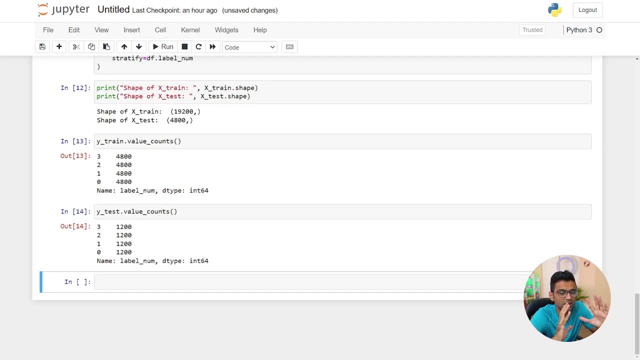 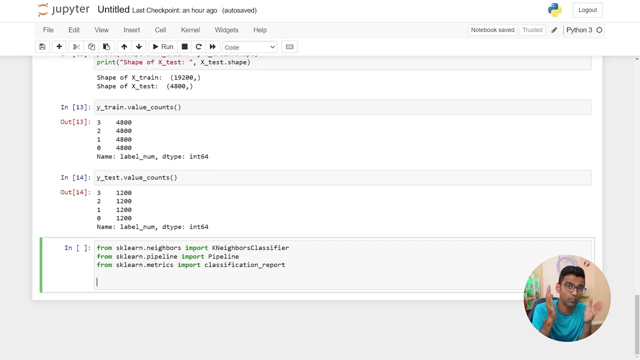 naive base. I just want to show you if you use different classific classifier, what is the performance. okay, so I will just import some necessary libraries and folks. I'm doing copy paste. I don't want to type and waste my time because we have done this enough number of times in this particular playlist, so make sure you follow this playlist. 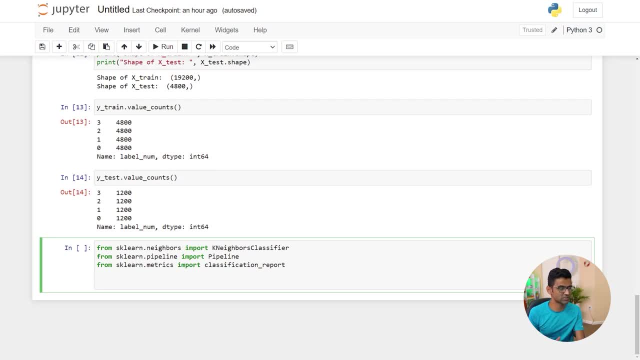 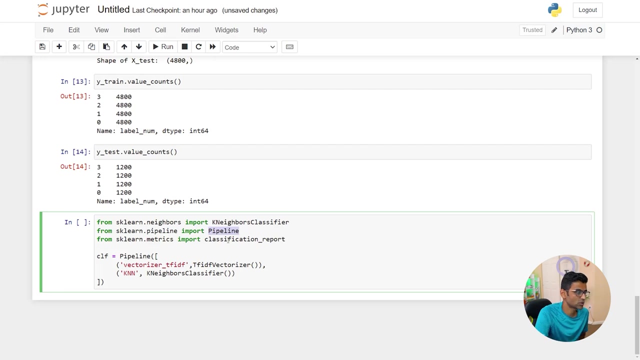 in a sequence. if you're randomly watching this video, some of these things might not make sense, but if you follow the playlist in sequence, it will be more meaningful. we'll import sklan pipeline, and sklan pipeline allows you to create a pipeline where, in the first stage, you can have 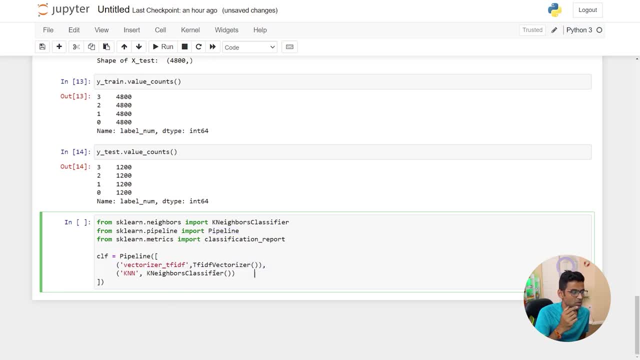 your tf idf vector and the second stage. you have your knn classifier and then you know you'll do clffit. so x train, y train, and then you do prediction right. once the model is strain you will say: predict x test and once you get your y predicted you want to. 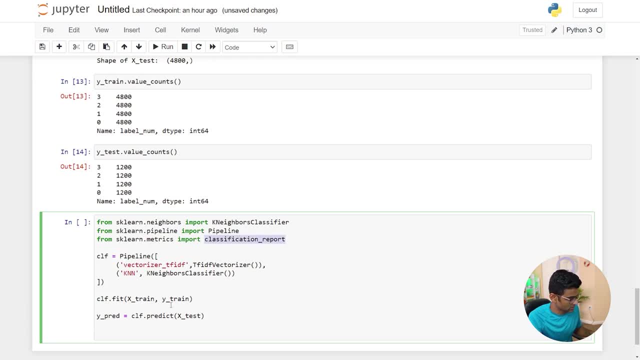 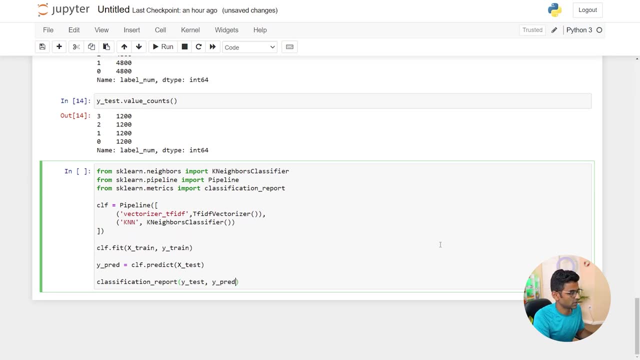 compare y predicted with your y test. and the way you do that is by printing classification report, and you always supply truth first and then the prediction, and I usually use print because otherwise the formatting won't be appropriate for classification report. so right now it is training the model in this fit command and then in the predict command it will do prediction on the. 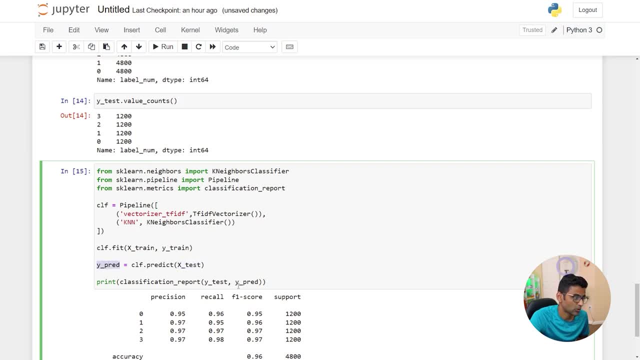 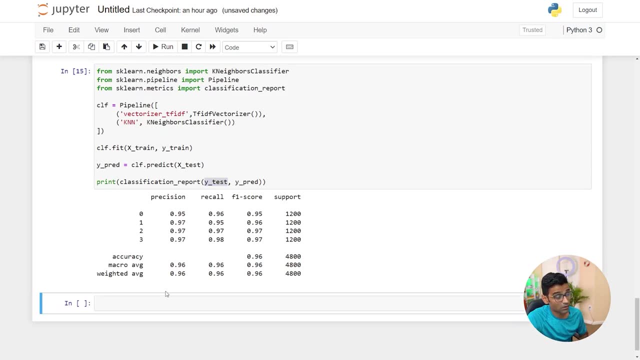 x space data set. it will get y predicted output and y predicted. it will compare it with the actual truth and based on that it has printed this classification report. the result looks pretty good. these are the precision and recall metrics for class 0, 1, 2, 3. okay, we know all those classes- household, books and so on- and these are the f1. 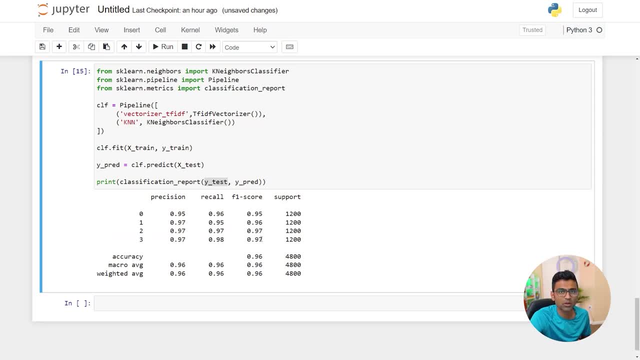 score: see f1 score of 95 96, 97. this is pretty good. if you don't know what is precision recall, go to youtube search code- basics, precision recall. you will find a video, very easy video, which explains all these metrics and I will just print. 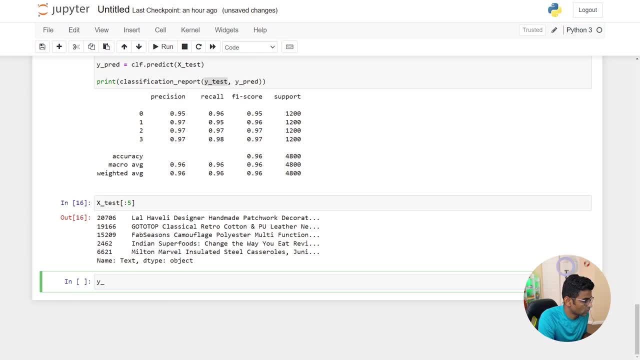 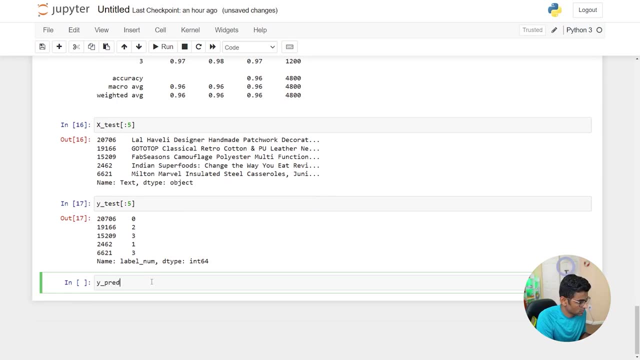 x test and what was my y test for first five sample? okay, and I want to also know my y prediction for first five samples. and see: zero, two, three, one, three. zero, two, three, one, three. only this one. it got it wrong. other categories it predicted fine, okay. so zero to category love Haveli. designer hand. 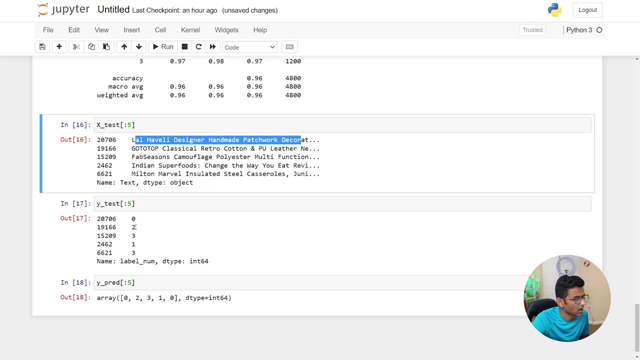 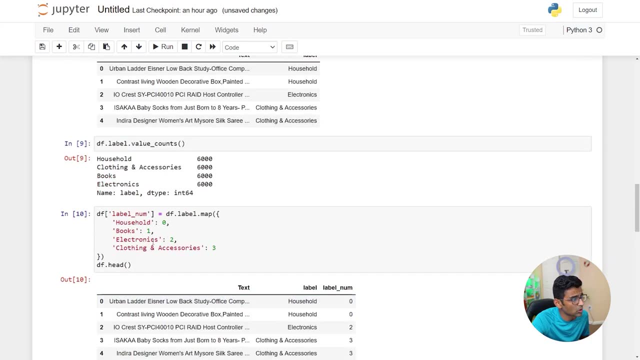 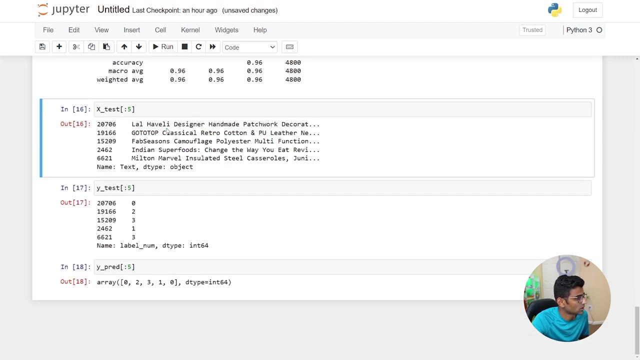 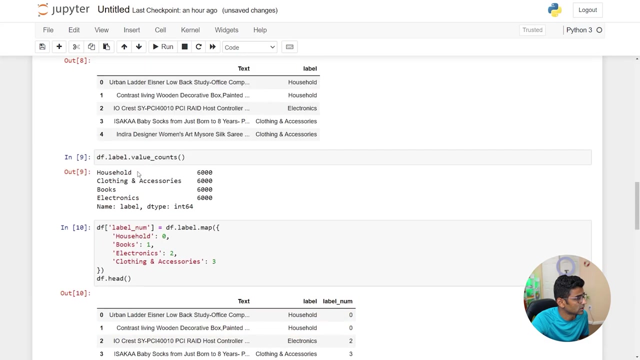 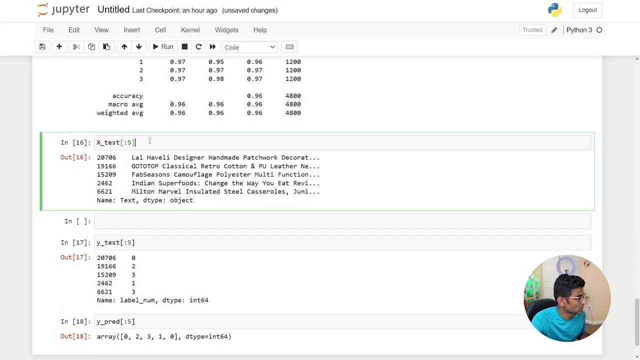 man, this looks like clothing item to me. household, so that is zero and you can see that household is zero. books is one, electronics is two. right, so this cotton thing, for example, go top, classical retro cotton is two, and two category is electronics. okay, so electronics, it is predicting it fine sometimes if the level is not clear. what you 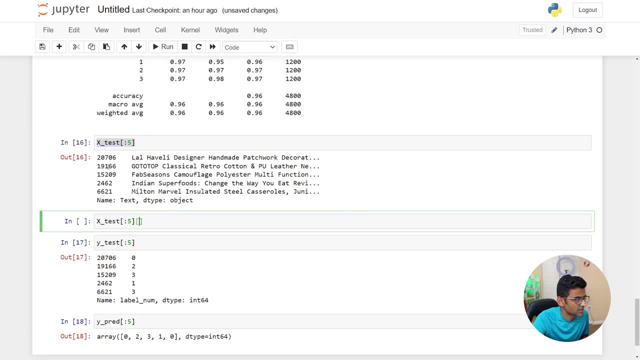 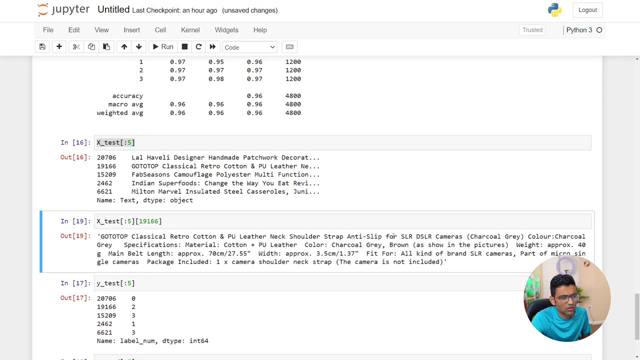 can do is you can print the whole thing and you need to supply this index. okay, this is the index that will give you the holes. see, you're talking about DSLR cameras, right? electronics? maybe this is leather, so maybe it's some kind of case for the camera. I don't know. 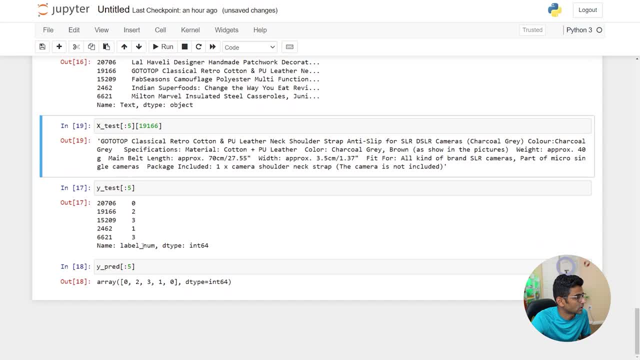 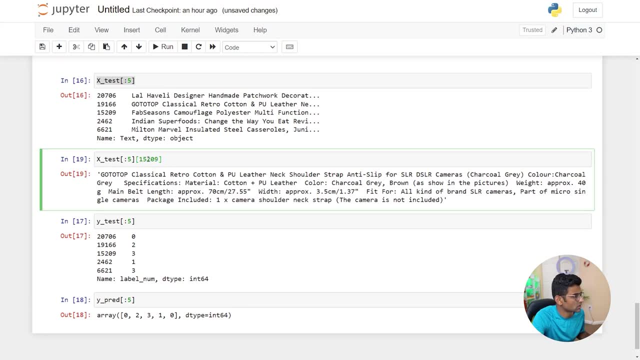 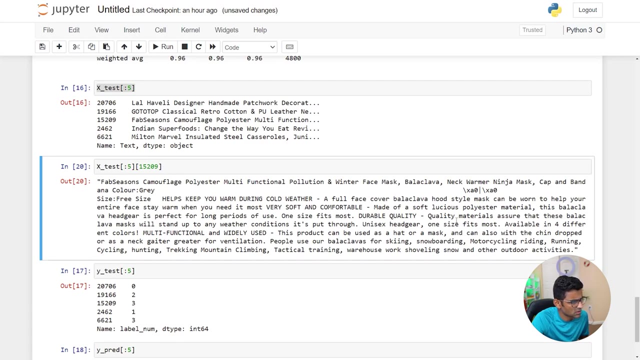 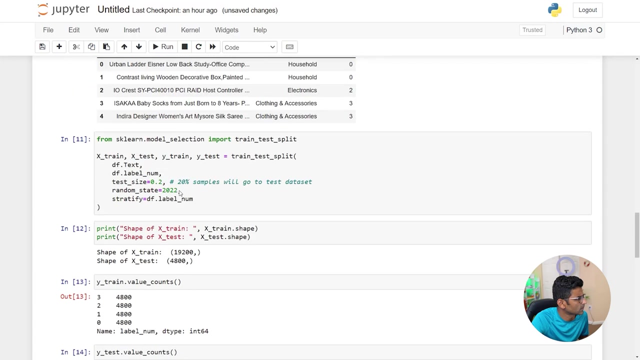 yeah, but anyway it is classified under electronics category. the third one is: see. the third one is this one, right? so this one is for, let's see, camouflage polyester multifunction winter face mask style mask. this is some mask, so household item. so number three, oh, number three, okay, sorry, clothing and necessary. numbers three is clothing and accessories. 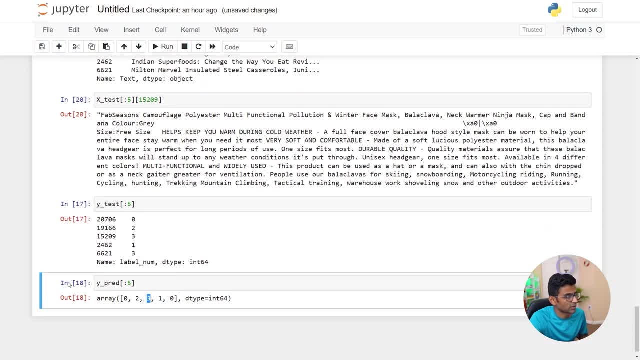 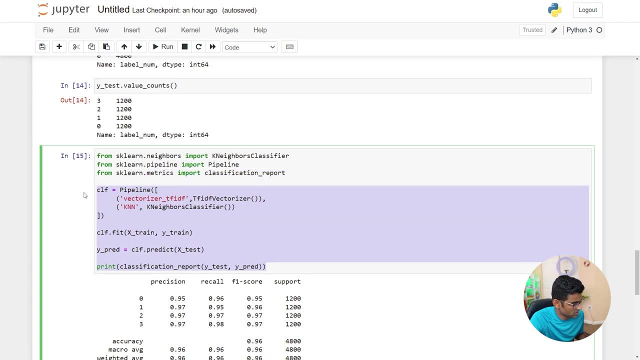 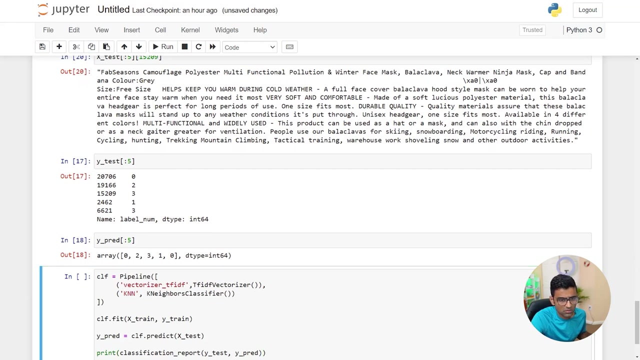 so the y test was that and prediction was also in in line with the truth. now I will use multinomial classifier as well and check the performance, so you can just copy paste this whole thing here, okay. and one additional thing you need to do is your naive base classifier you need to import. 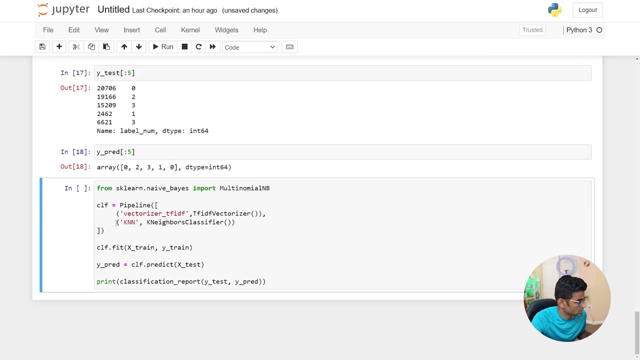 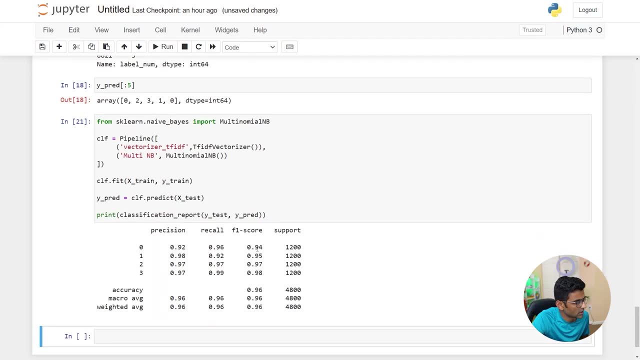 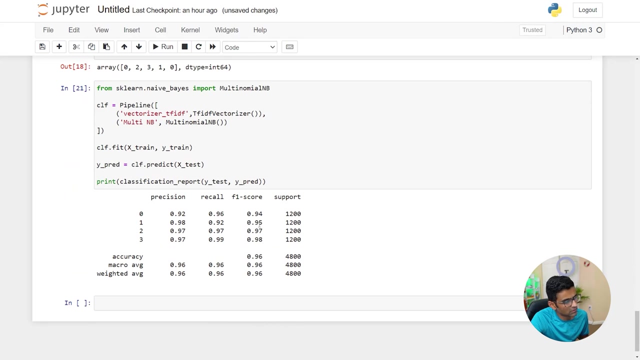 and use that one here in the second stage of your pipeline. here you want to check how the performance looks like and you compare. so see here: K and N give 95, 96, 97, 97, 94, 95 97. almost similar, okay, not too much different. but now I want to try. 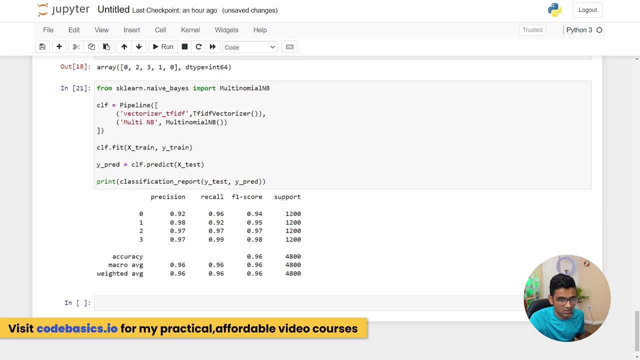 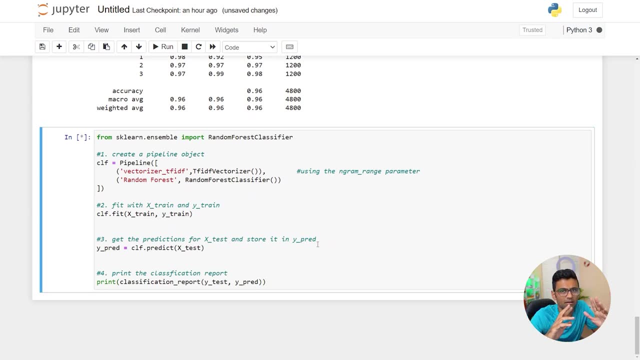 a random Forest classifier. okay, so I will do random Forest classifier and you can see this could be trial and error. usually for text problems, you see that something may be not right or it will could be a trial and error, so you can check and compare. okay, in the first instance, let me check this once again, bernie, here was what is your error? from a率 to Gamma and so on? what was your Зап d Pretzel? 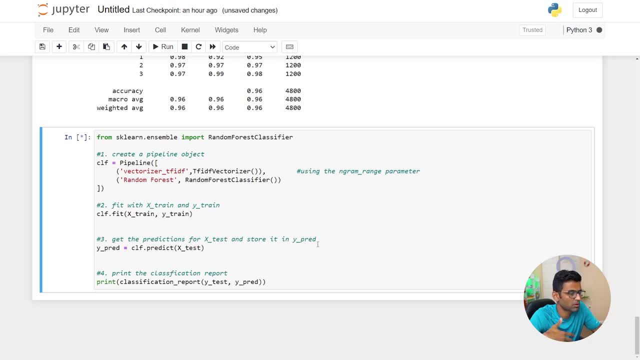 I start with naive Bayes. but based on your problem, your data said you know one or the other classifier might perform well, there are some general guidelines you can follow. okay, test classification: usually use multinomial naive Bayes, but in this particular case what's happening is see random forest is giving you. 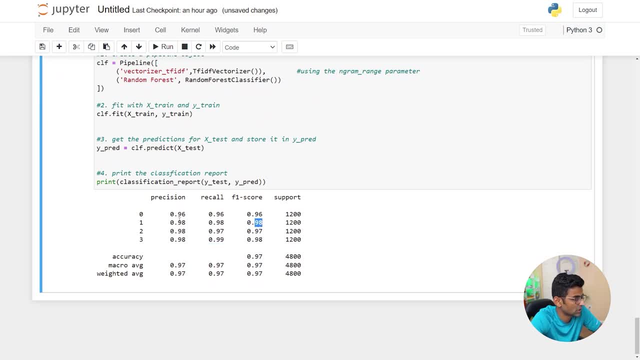 probably the best performance: 96, 98. you can compare all these metrics with these, these other metrics from the other classifiers, and we concluded that the random forest classifier is giving you the base performance. now, when I train this model, I did not do any pre-processing, I did not remove, stop. 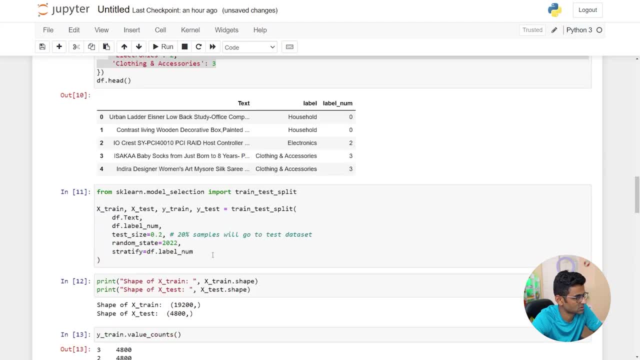 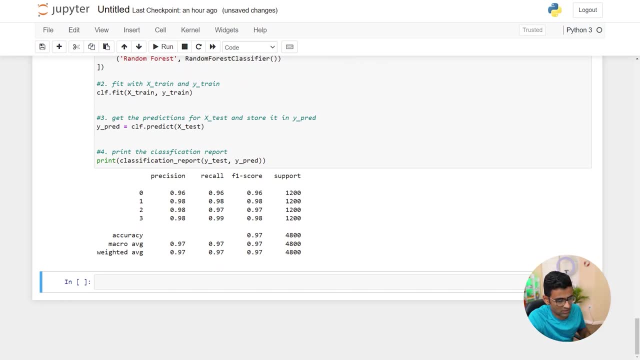 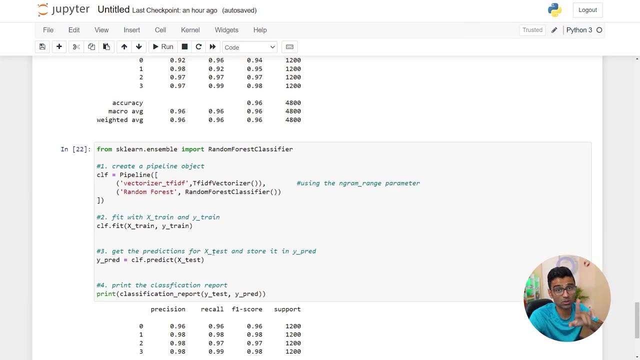 words and I did not do lemmatization. so remember, in the last tutorial we we designed a function that can do this- pre-processing, so I will do that now. I will train this same classifier, but using pre-processed text, not the raw text. this classifier is: 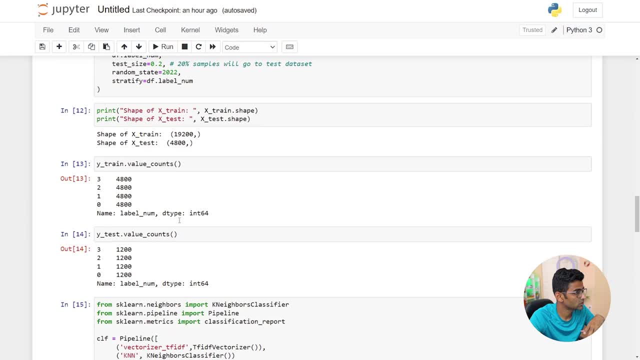 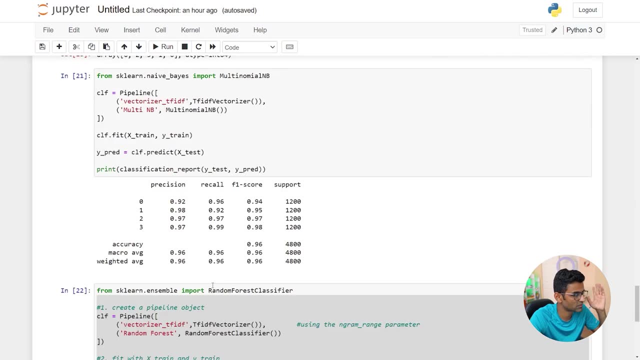 trained on a raw text. how do you know? well, see, we use in train this place df dot text. df dot text is whatever we got in our CSV. we did not remove stop words or we did not do lemmatization. I want to do that, so I will import a specie. 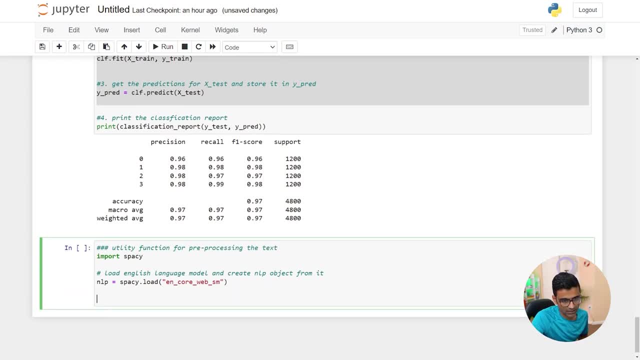 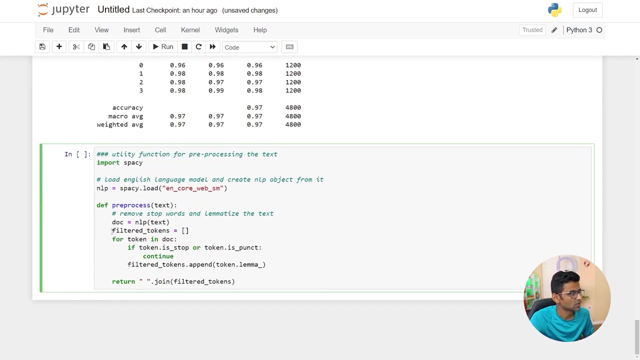 library and I will define a function called pre-processed. now we have seen this exact function in the previous video and here we need to do this in our IV. I'm not going to use the pre-processing. let's say it's a simple composition in HeyPier. if we want to do 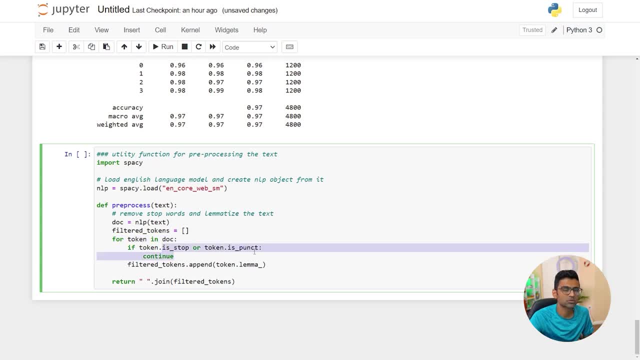 long term. you will use a Drame and instead of doing it in a short term, here we have a variable, we will be doing it in a long term. you can change this to method, or you can write a script, and we will do it in a similar way. since I'm 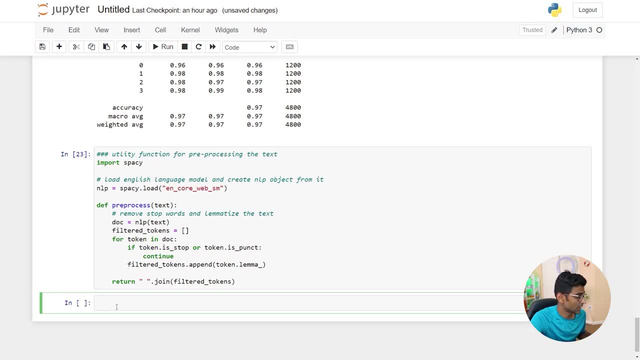 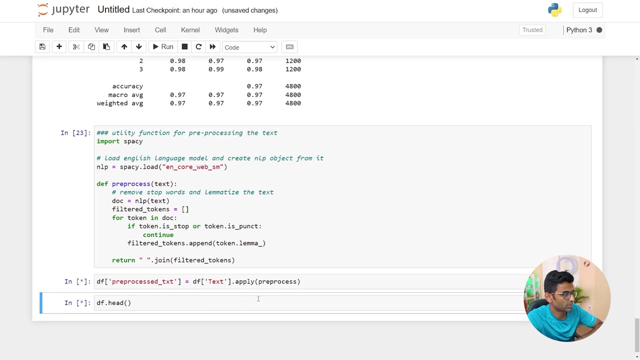 not going to go line by line. I will use my most powerful weapon of copy paste column. you will use apply function and use a preprocess apply and map that kind of similar function and this will create a new column called preprocess text. it took me close to 10 minutes. 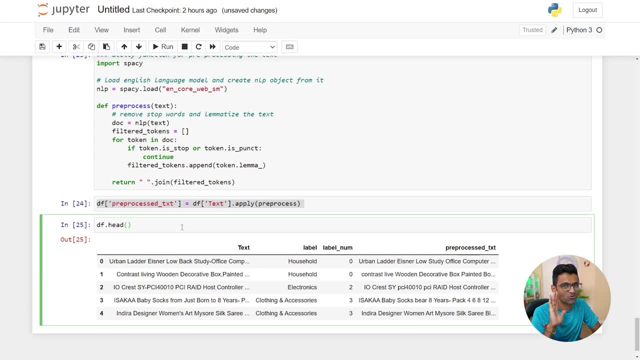 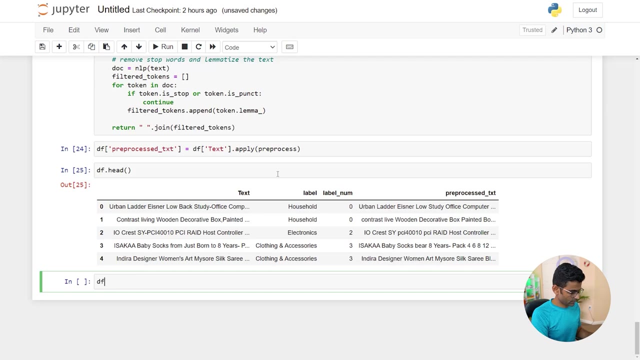 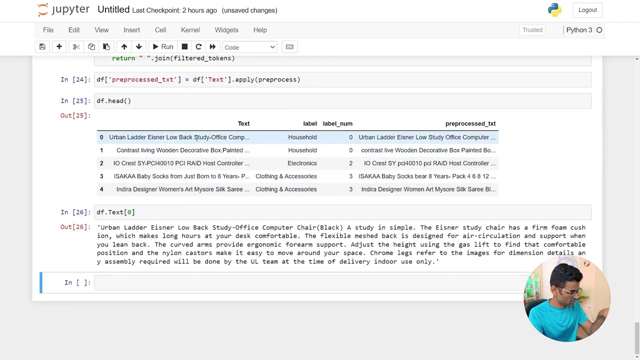 to execute this sentence, so make sure you have enough patience. you go for a coffee break or a walk while this is executing, and I got this new column created and this has a preprocessed text, so let's check one or two specific examples. for example, the zeroth text right, the zeroth, the first. 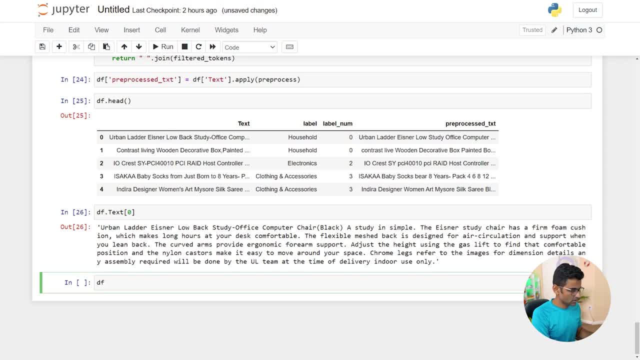 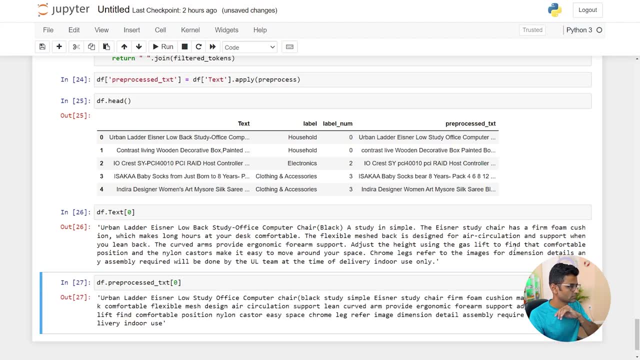 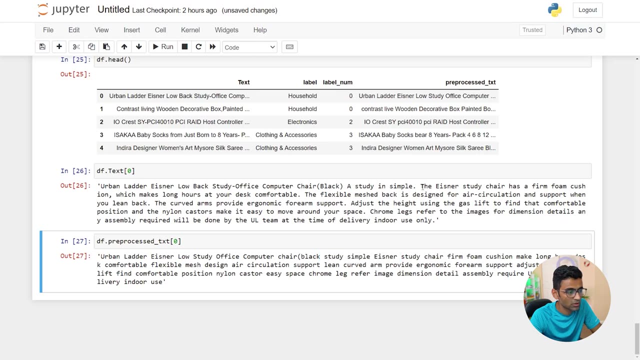 one is this, and if you look at the same thing in preprocessed text, you you will find that see a study in simple see a study is in is removed, the is removed, punctuation dot is removed. see here then chair has a firm. it will be said: chair, firm has a firm is removed. so it got. 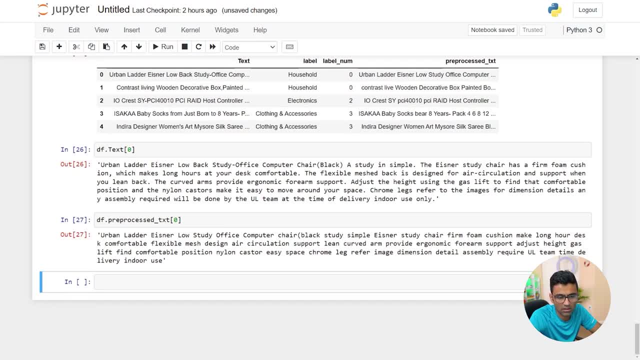 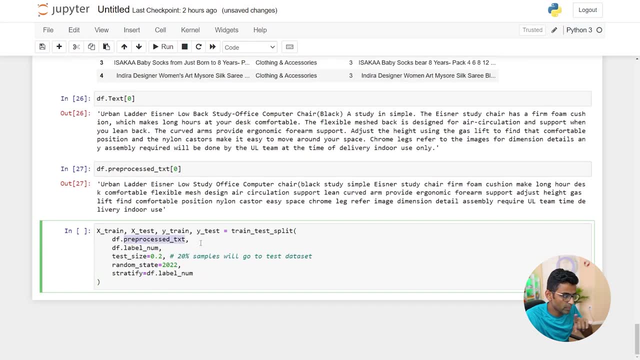 rid of stop words and some, and it did lemmatization and so on, and we'll do the train test split using the preprocessed text column. here again, the random state is same. because of that, the- the samples that we got in the previous scenario where we are using our nateks, built that similar so that we can do apples for comparison. 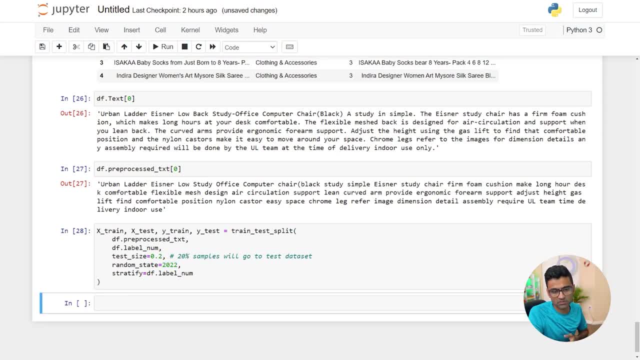 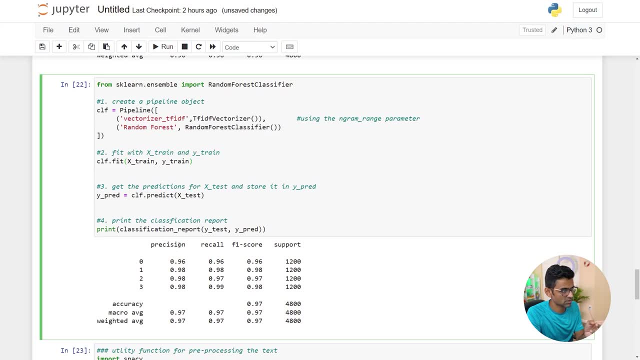 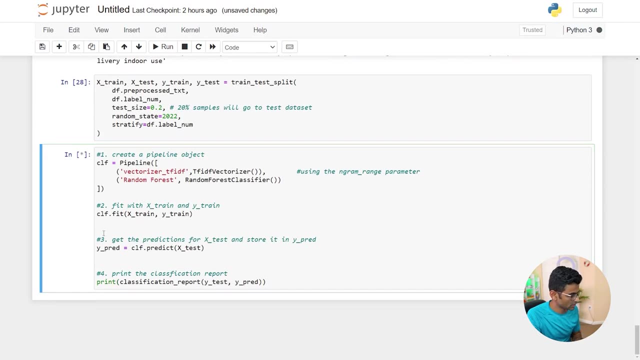 when we are doing this prediction and I am going to copy past the same call for random forest back from here. get the same code I was just copied and pasted, which is my most powerful weapon, and then I have. when that is finished, withPUT and I will train the model. this model is trained using preprocessed text, the. 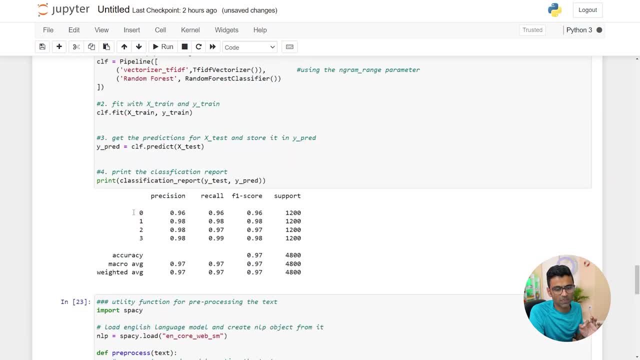 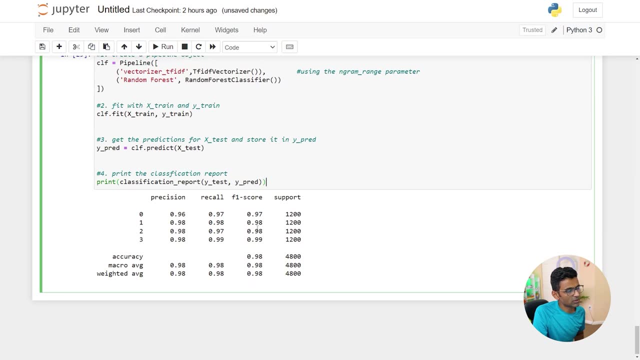 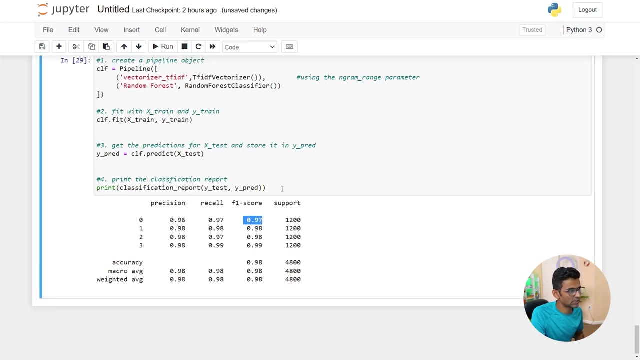 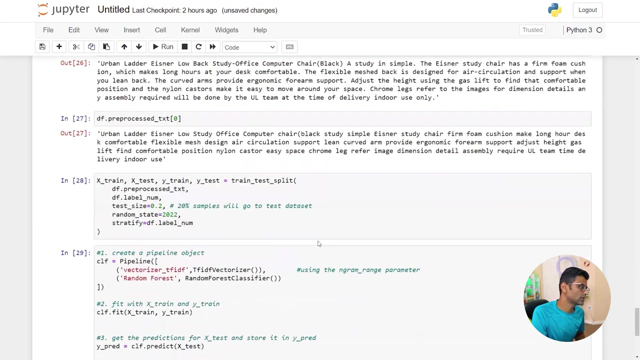 numbers that you saw above. these are using the raw text and you will notice the performance is slightly better. so f1 score 97, 98, 98 and 99 correct here. see it's little less when you use raw text. so we can conclude that in the case of 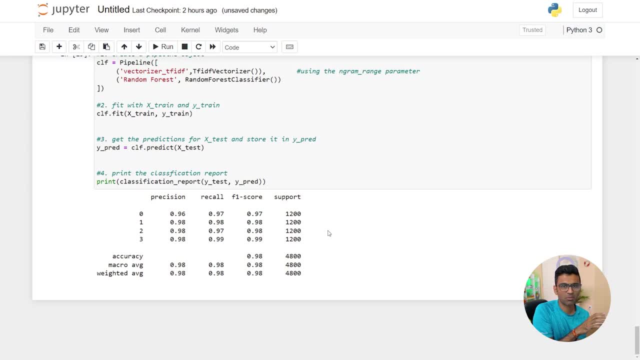 this e-commerce classification problem. with this particular data set, the preprocessing is helping. general guideline is: you should do preprocessing, but in some cases, if you don't do preprocessing, it is still okay. so it just varies from case to case. I hopefully you like this video. this is